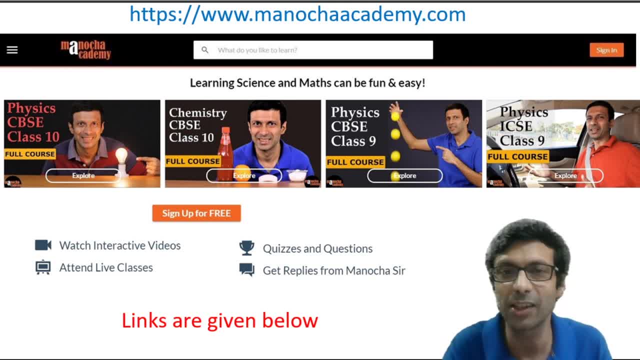 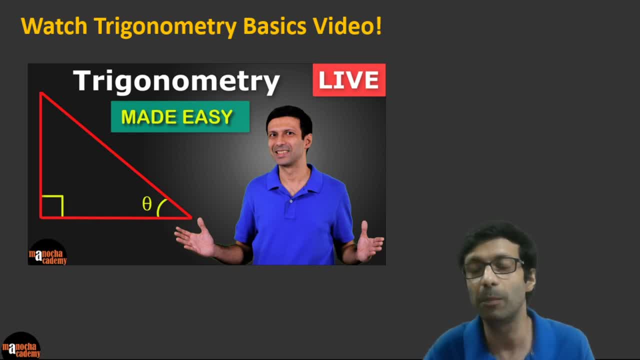 And if you haven't hit the like button, please hit the subscribe button. And if you haven't hit the subscribe button right now, and click on the notification bell so that you don't miss out on any videos And guys, if you haven't seen the trigonometry basics video, then do check this. 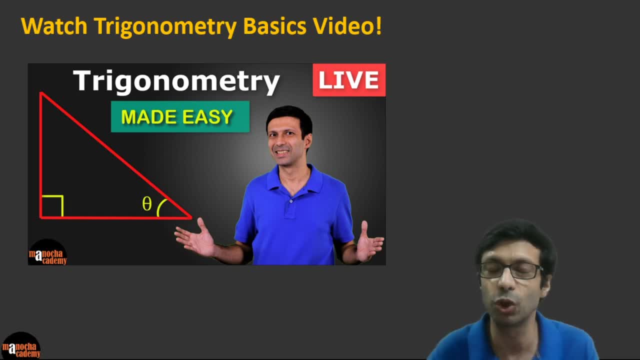 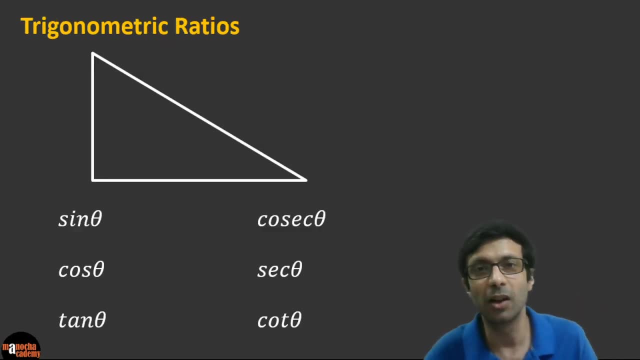 video out. I've uploaded it on our YouTube channel, Manocha Academy, So do watch that. Alright, guys. so good evening everyone, and great to see all of you here. So welcome to this maths class and let's look at trigonometry. So, guys, as you know, in trigonometry 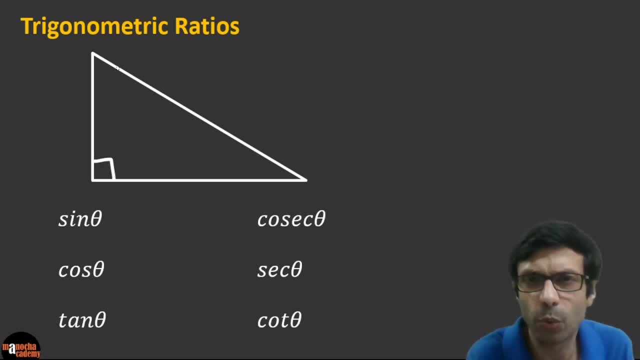 we need a right angle triangle, right? So let's quickly revise the basics. So this is a right angle triangle, ABC, right angled at B, And let's say this angle is theta. Okay, so this is the angle theta. then what are the trigonometric ratios that we can define? So, guys, you know that. 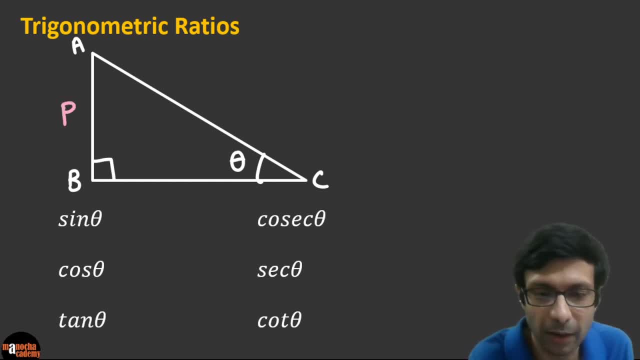 this is going to be the perpendicular which I'm showing in pink color, the base here right. So for this angle, theta, this opposite side is the perpendicular. This BC is the base because it contains both the 90 degree and theta And the side opposite to the. 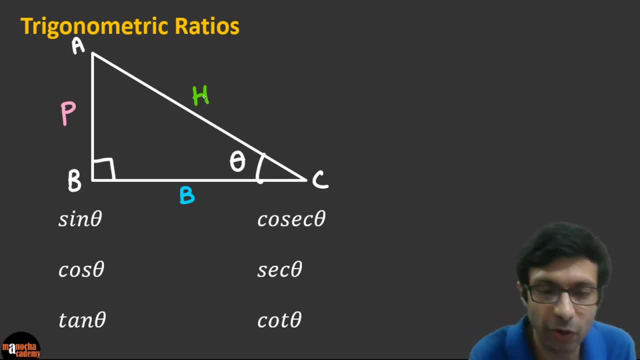 90 degree is called the hypotenuse. So now we can take a ratio of the sides and we can define these trigonometric ratios. So you know that perpendicular by hypotenuse is sine theta, right, guys, And guys, what is cos theta? So cos theta, guys, is base by hypotenuse, right? So base. 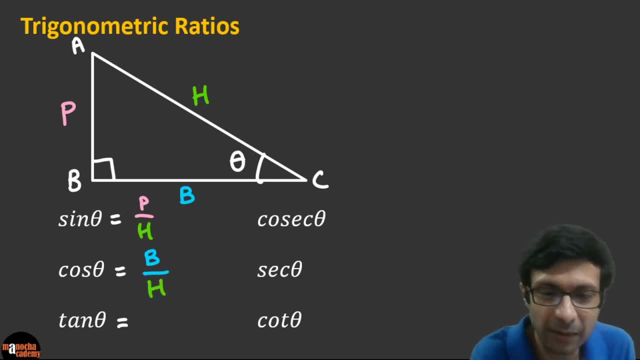 by hypotenuse. And what is tan theta? You guys know tan theta is perpendicular by base, okay, So make sure you learn all these trigonometric ratios. And what is cosec theta, Guys? you know that these, what you see on this sides, are the reciprocals, right? So cosec theta is. 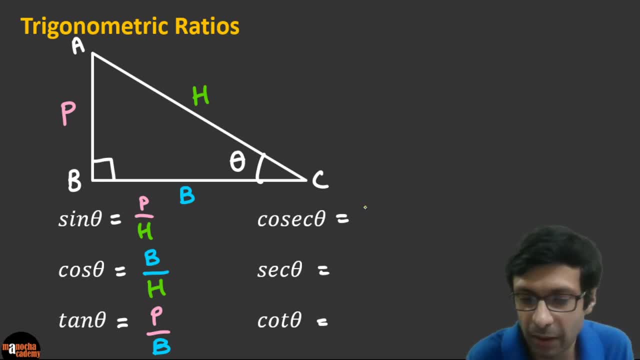 one by sine theta. So we can say it's going to be hypotenuse, right? So this hypotenuse divided by the perpendicular, because it's the reciprocal of sine theta. And, guys, what is sec theta? So sec theta is going to be: 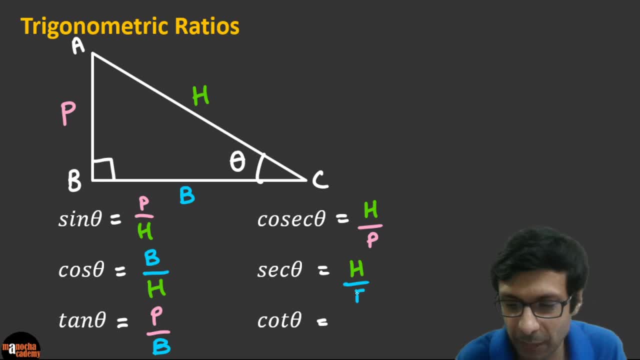 hypotenuse by base right And cot theta is the reciprocal of tan theta. okay, So can you see, we need to invert P by B, So it's going to be base by perpendicular clear And please remember this is only trigonometric ratios are taken for a right angle triangle And, as you can see, 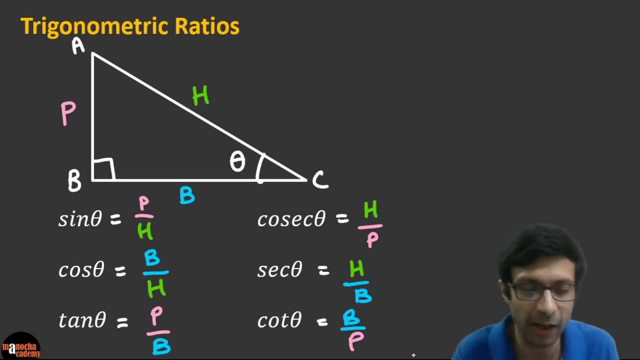 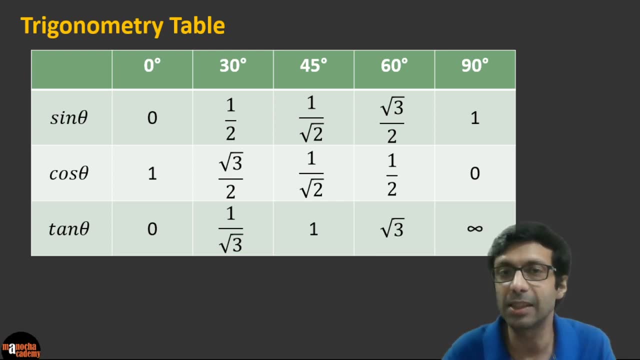 we have taken them for this angle theta, or you can call the angle A or X right, And we also looked at this table in the last class. You need to learn up these standard, important values of sine theta, cos theta, tan theta. 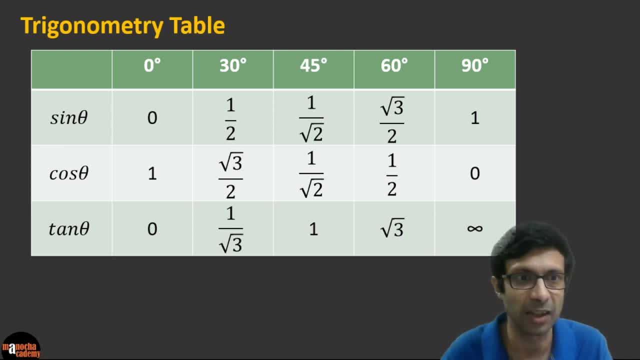 right For 0,, 30,, 45,, 60, and 90 degrees. So, guys, make sure you know all these values, because they are very useful in the sums, okay, So do learn them up. So now in today's class, 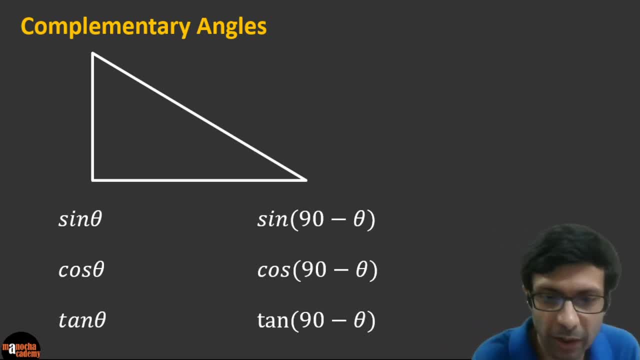 we're going to look at something called complementary angles, okay, So again we have this right angle triangle right, Which is right angle at B here, as you can see, guys. So ABC, and let's take this angle, theta. okay, So we are taking this angle, theta, So let's write. 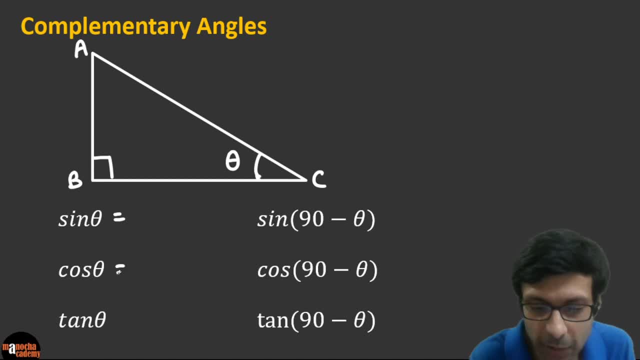 down. so what will sine theta be? So let's quickly write these in terms of the sides. okay, So sine theta, right? Remember we said it was perpendicular by hypotenuse, So here sine theta is going to be basically the perpendicular. here is A right, So sine theta is going to be perpendicular by hypotenuse. 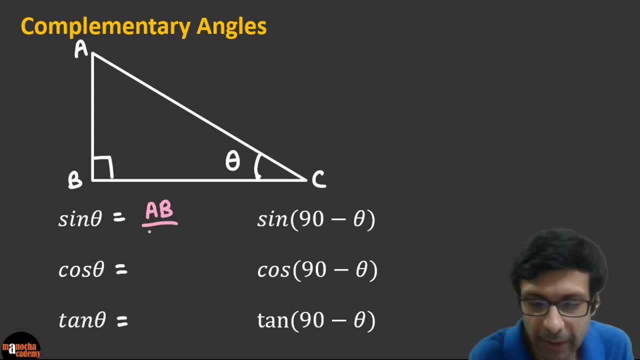 AB for theta. So it's going to be AB by AC right For this triangle. what is cos theta going to be guys? So cos theta for this triangle is going to be the base BC right. This is the base divided by the hypotenuse AC right And tan theta guys is going to be. can you see that? 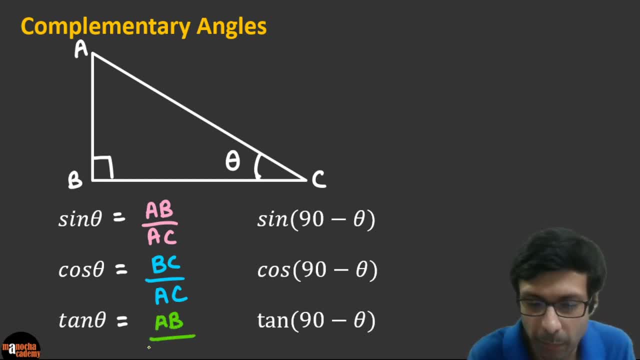 AB, the perpendicular by the base, which is BC here, right? So did I get my ratios, right, guys? So this angle here is going to be 90 minus theta, right? So these angles, so the angle A and C, are complementary because they add up to 90 degrees. Let me write this a little more clearly. 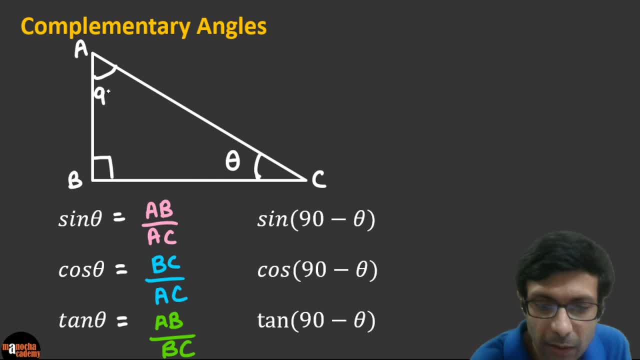 for you. So this angle, can you see, is going to be 90 minus theta. So can you see, guys, here the angle A and C are complementary because they add up to 90 degrees. So this angle, can you see. 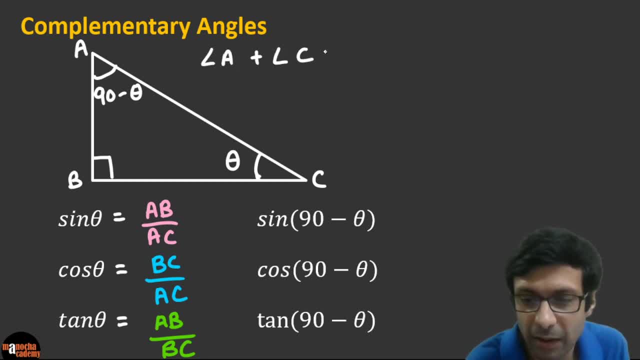 plus angle C is 90 degree, right, Because it's going to be 180 minus this 90. So these two angles need to add up to 90 degree so that all the angles in the triangle add up to 180.. So now, 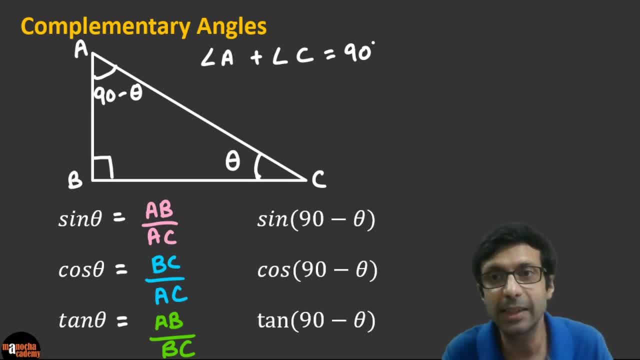 if you look at the trigonometric ratios of 90 minus theta. okay, Okay, Some of you are asking what is meant by theta. So good question. Theta is basically just a symbol right that we use for denoting the angle. So if you look at the trigonometric ratios of 90 minus theta, 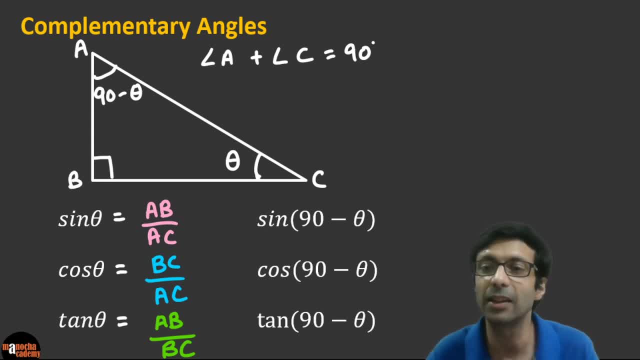 the angle right, So this is a variable. right, This angle theta, so the angle in this triangle, theta can be, take the value of 30 degree, 40 degree, 45,, whatever right, So it's a variable. 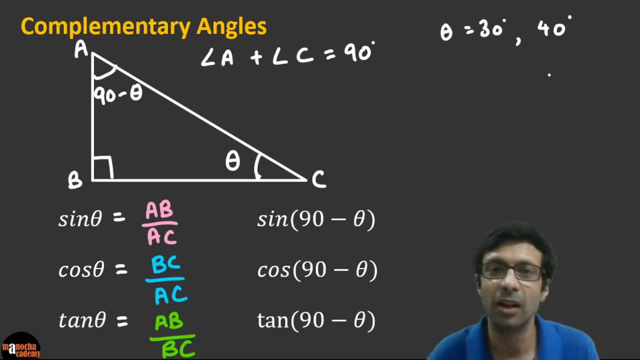 just like we take x in algebra, Or you can even take, we can say sine of C. okay, So rather than writing theta, we can say sine of C or sine of x, But usually in trigonometry we use, we mark the. 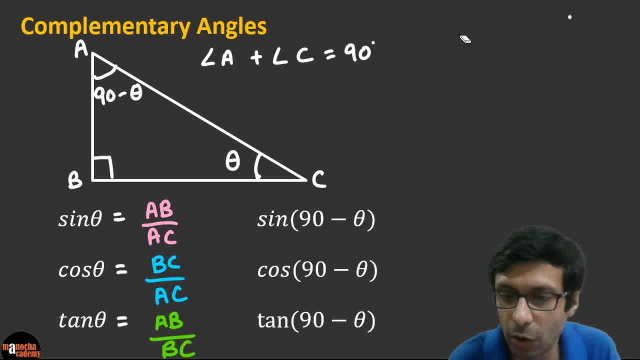 angle as theta. okay, So now let's take a look That what is sine 90 minus theta can be is going to be. So, guys, can you tell me here, So can you help me out, What is sine 90 minus theta going to be in terms of the sides? So what? 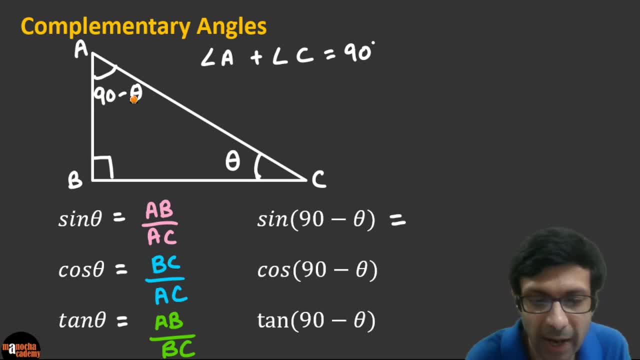 is the sine of this angle going to be The angle A, which is 90 minus theta. So who can tell me? what should I write here for sine? 90 minus theta. So this one right? Okay, First, tell me in terms of the sides. So I'm not asking, so in terms of the sides. 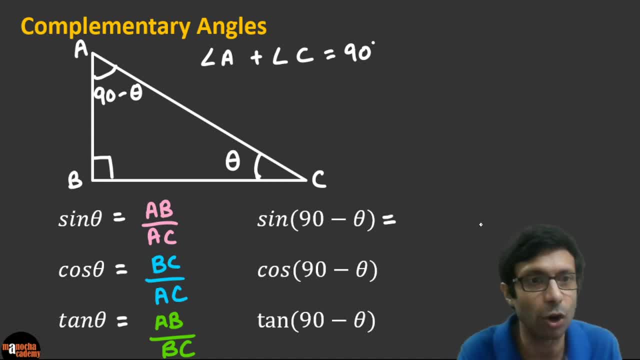 it's a trigonometric ratio, So should it be AB by AC or should it be something else? What do you guys think? Okay, So, very good, I see some answers there. So if you look at this, 90 minus theta, sine of 90 minus theta is basically going to be the perpendicular by hypotenuse right. 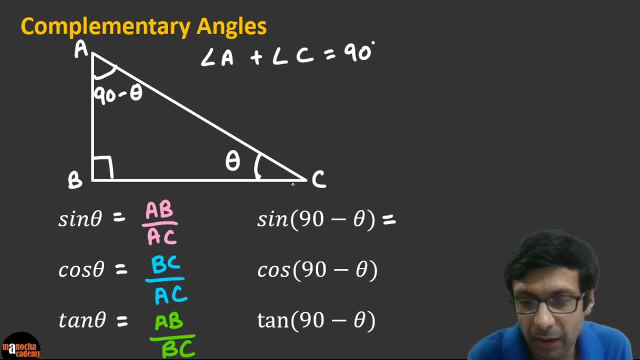 So what is the perpendicular for this angle? It's going to be this side, right. It's going to be now BC, not AC, because the side opposite 90 minus theta. So it's going to be BC by the hypotenuse, which is AC Clear. So let's write. 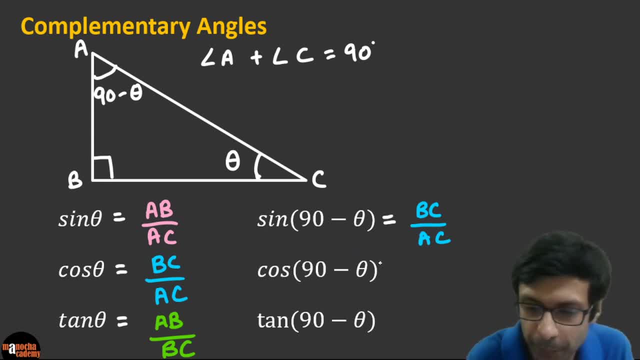 that down. Similarly, let's write it for these guys also. So what is cos 90 minus theta going to be in terms of sides? So let's get the concepts really clear. Okay, So cos 90 minus theta, can you see? So for this angle, A 90 minus theta. cos 90 minus theta is going to be base by hypotenuse. 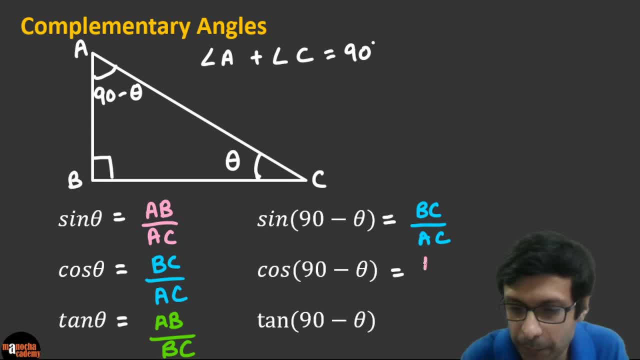 So what is the base here? The base is AB And the hypotenuse is again the same AC. So I'm going to write AB by AC. Very good, I see a lot of you said AB by AC. Excellent guys. And what is tan 90 minus theta going to be? So you know, tan means perpendicular by base. 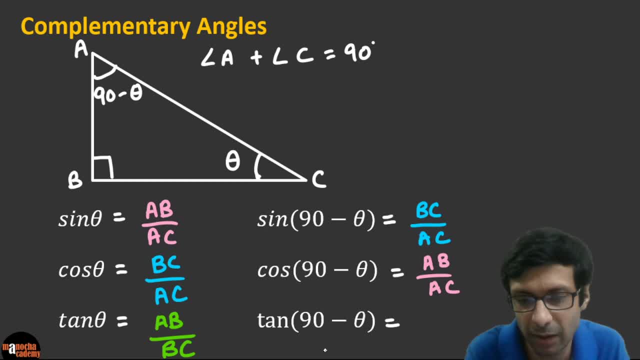 So let's look at who's the perpendicular and base for 90 minus theta, right? So for 90 minus theta it's going to be basically BC by AB. Can you see that BC is the perpendicular for it and AB is the base? 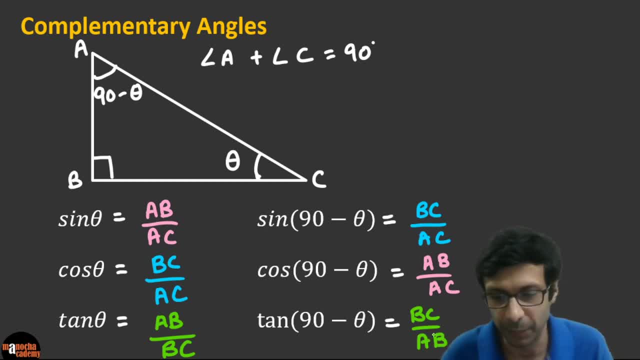 Right, So we've written these out clearly. Does that make sense? Right, Simple? So now let's, guys, let's go ahead and see what's the interesting connection here with these complementary angles. And can you see in the? I've used some color matching here, So maybe you guys. 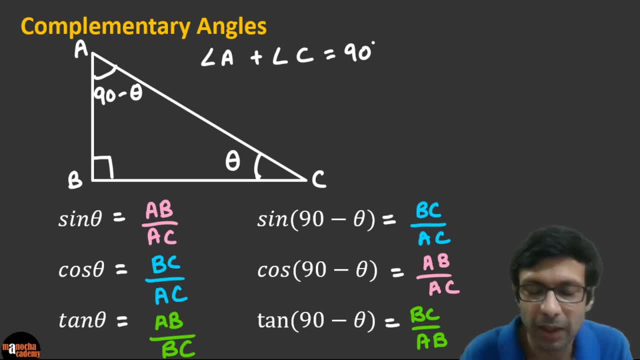 can see out here. So what do you think? What are the important formulas we're going to get for these complementary angles here? Let's take a look, Okay, So basically we'll have cos 90, minus theta- All right, Sorry, sine 90 minus theta. Let me start with the first one. So let's erase this thing here. 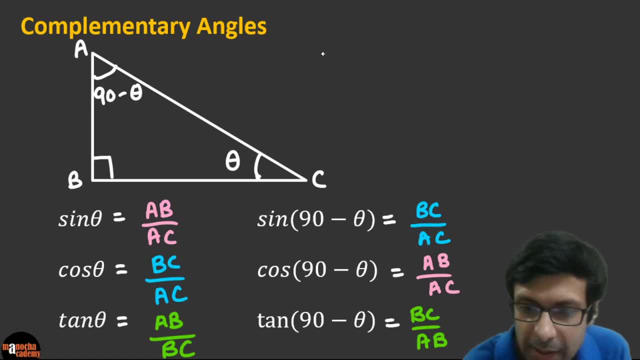 Right. So we are basically going to have sine 90 minus theta. right Is so sine 90 minus theta is BC by AC And can you see that's going to be equal to cos theta. So this is a very interesting relationship. 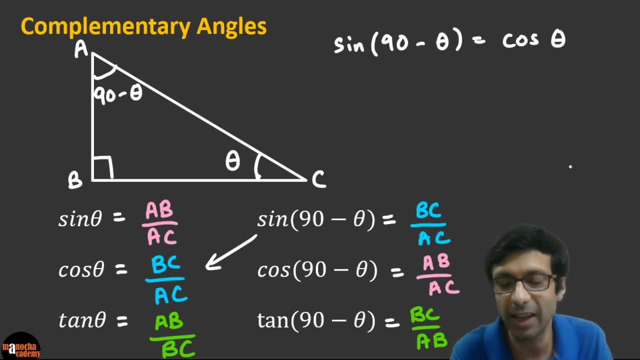 for the complementary angles: theta and 90 minus theta. So sin 90 minus theta, right, So that means 90 degrees, right. So sin 90 degree minus theta is cos theta, Okay, very good. Similarly, we will get guys, what do we get for cos? So excellent guys. So what will cos 90 minus theta? 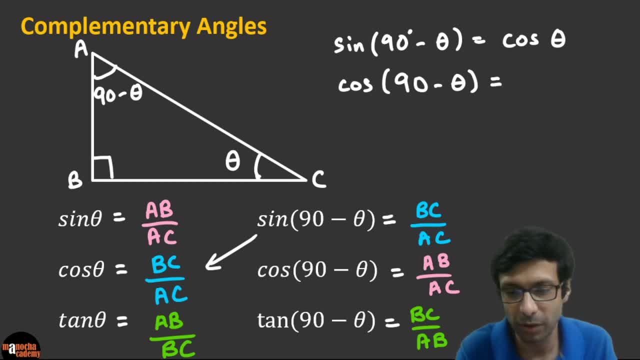 be. Can you guys tell me by looking at these trigonometric ratios: Okay, So here we saw that these guys were related, right? So these guys were the same, right, BC by AC. And what will this guy be? Very good, Very good guys. So cos, 90 minus theta is going to be sin theta, You guys. 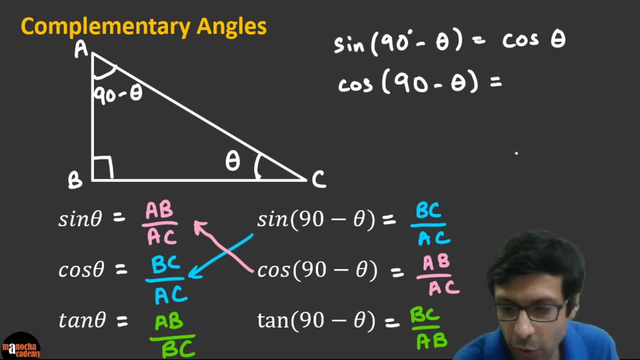 rock, absolutely right. So from this formula can you see, If you compare cos 90 minus theta, it's same as AB by AC, which is going to be sin of theta. So we are getting some really interesting formulas. And what is the connection between tan 90 minus theta? 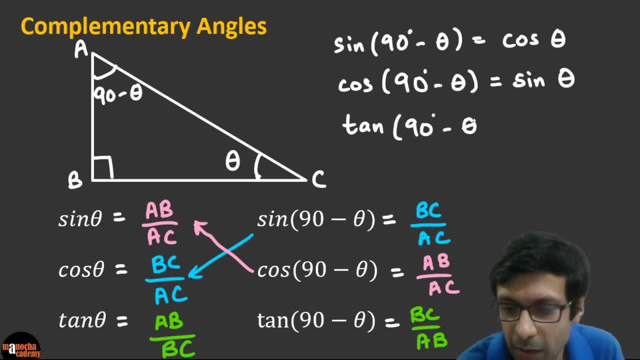 right. So tan 90 minus theta- Is that equal to tan theta, or what is it? What do you guys see there? Okay, So can you see that tan 90 minus theta is BC by AB and tan theta is AB by AC. So 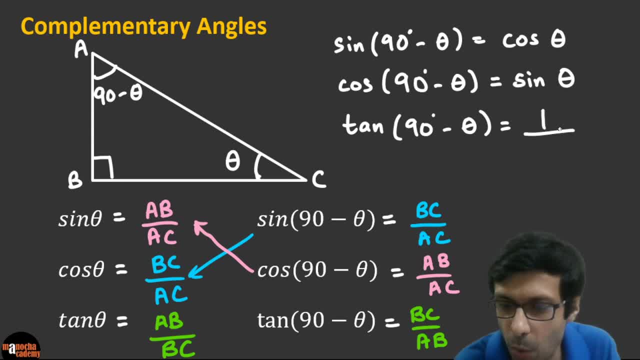 they are reciprocals of each other, right? So this is basically 1 by tan theta, Or I can write, you know that 1 by tan theta Very good, Excellent Is cot theta, Superb guys. So 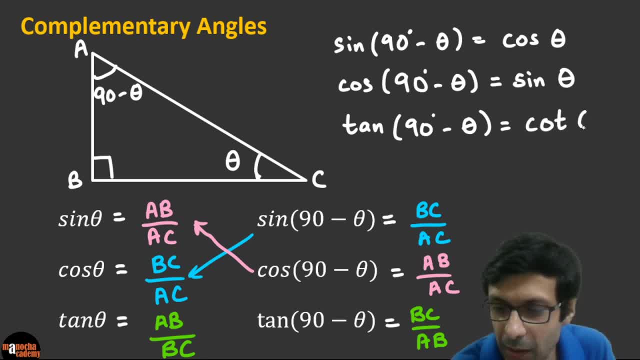 this is the formula. It's basically 1 by tan theta, which is basically cot theta. So these are very, very important formulas for you to remember: Sin 90 minus theta is cos theta, Cos 90 minus theta is sin theta And tan 90 minus theta is cot theta. So can you. 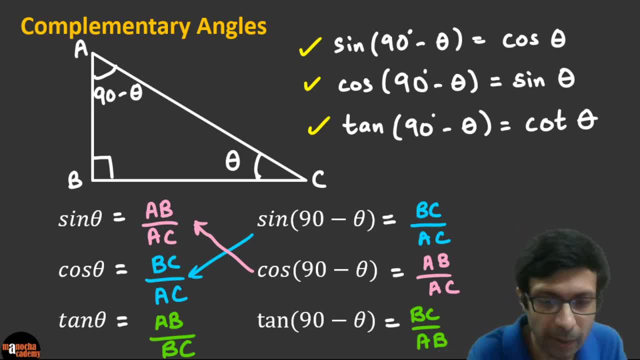 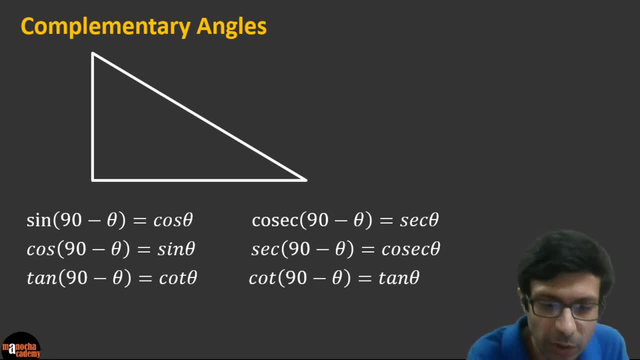 see how the complementary angles are related in this interesting way, right, And we can use this in our questions. So these are the formulas, right, And similarly you can also. so we just looked at these formulas for the right angle triangle, right? So ABC here, right, This was. 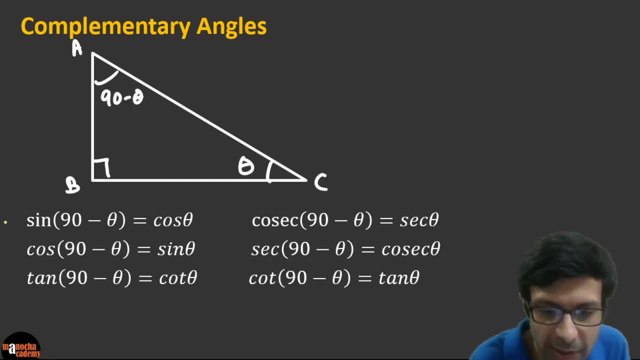 our 90 minus theta. And we learned these important formulas right Just now. we looked at these And if you take the reciprocal right, So it's going to be cosec, because you know that cosec theta right, You guys know Cosec theta is basically 1 by sin theta, right. So from here we can say: 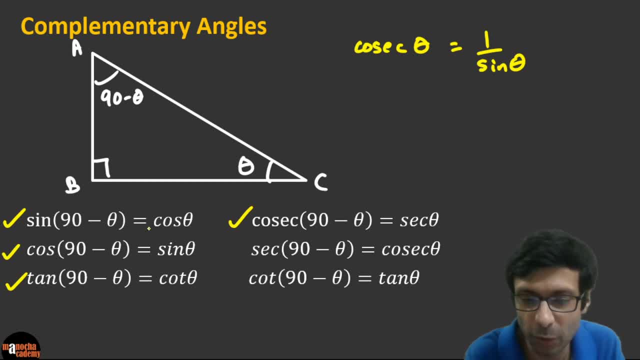 that if you take the reciprocal cosec of 90 minus theta is going to be sec theta because sec theta is going to be 1 by cos theta. Simple right. You guys know these And similarly you have from this relation. you can get the next one Sec of 90 minus theta is going to be cosec theta And similarly. 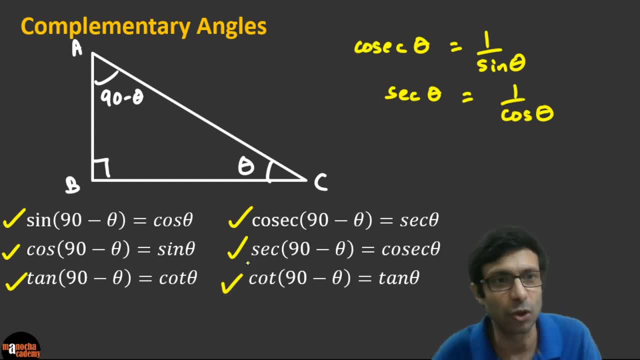 if you take the reciprocal cot of 90 minus theta, is going to be tan theta, Okay. so just absorb these formulas And guys. the best way to learn them is to write them down. Don't read the math book. you know, like a storybook, like a Harry Potter book, right, You need to write down these. 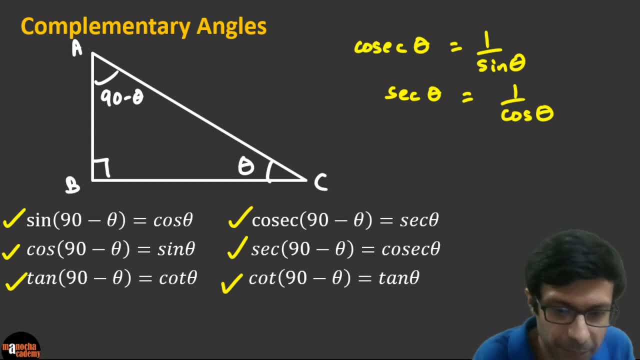 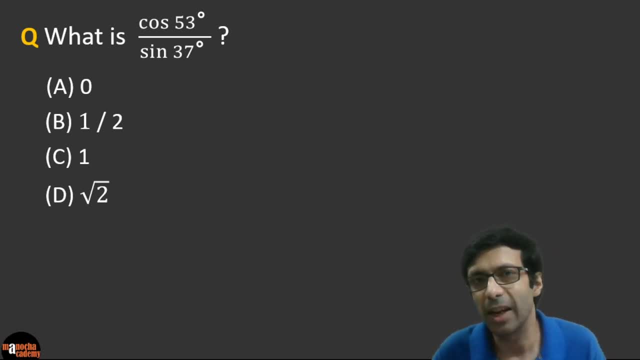 formulas, then you'll absorb them. Okay, excellent, Right, So now let's take a look at this question. So can you tell me, guys, by using what we've learned so far, what is cos 53 degree by sin 37 degrees? 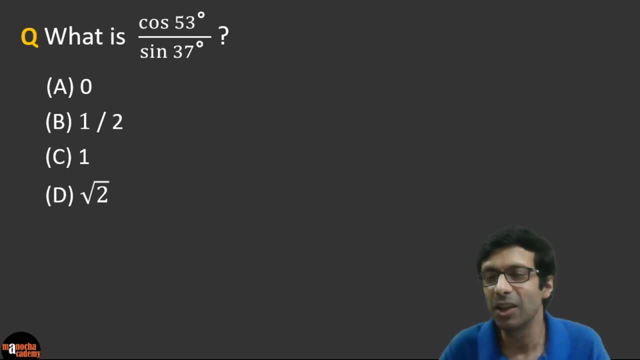 Okay. so, guys, I want all of you to try, And hint is: we've been talking about complementary angles, So what do you guys think this ratio is going to be? So I've been, I've asked you to find. 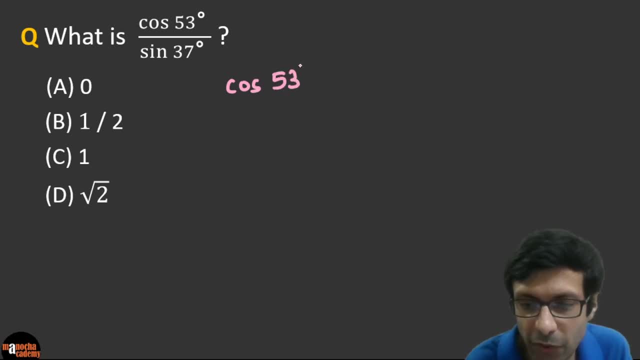 cos of 53, right Cos, 53 degrees divided by sin 37.. So, come on, who can tell me the answer of that? Wow, awesome, You guys already are writing the answer. You guys are really fast, Excellent. 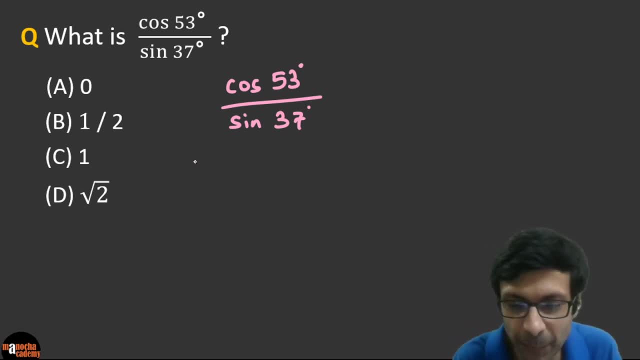 So let's see how to work out this question. Fantastic guys. So first thing, you notice here that if you look at 53 and 37, if I add them up, what do I get? 53 degree plus 37 degree. 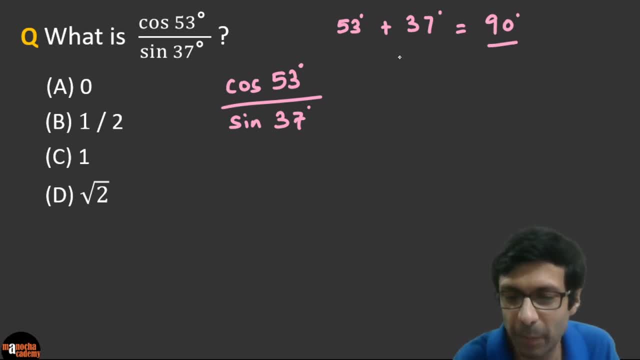 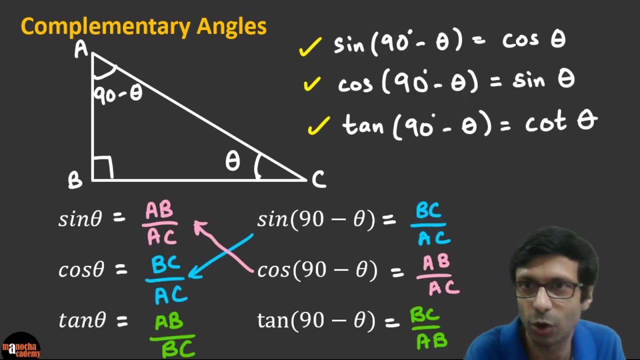 is going to be 90 degrees. Do you see that? So these are basically. so we have complementary angles, right, Because the definition is they add up to 90 degree. So basically, we can use our formulas that we learned right. We can use these formulas or the formulas we talked about here. 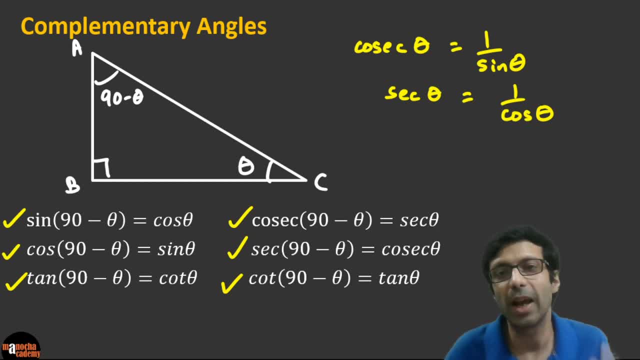 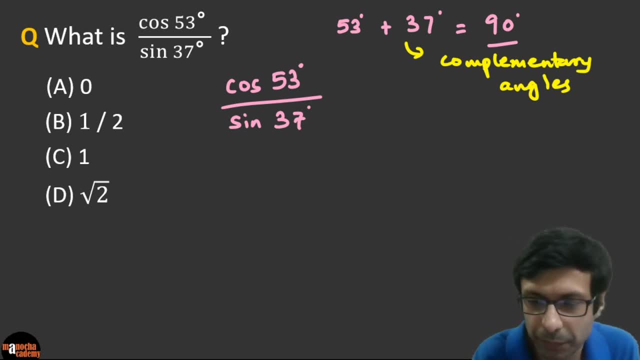 right. So, and we've summarized it in this slide, So we can apply these formulas to that question, Okay, So let's see how do we do that, Because we have these complementary angles. So, guys, what do you think we are going to do here? So, if you look here, we can write the first. 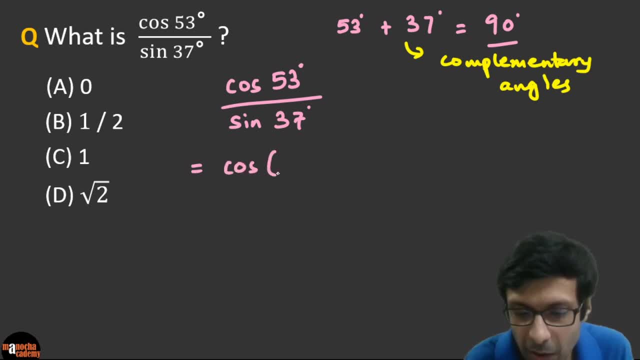 one. So cos 53 can be written as cos 90 minus 37,, right, Because 53 is 90 minus 37. And then let's write this down as sin of 37. Right, guys? Okay, So what is the trick? We are changing cos. 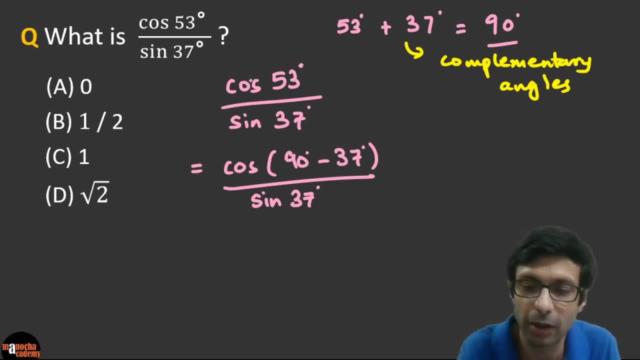 into sin. okay, Don't change both. Don't change the numerator Cos to sin and then denominator sin to cos, then you'll be nowhere, right? So we are changing one of them. So cos 90 minus 37 is going to change into sin of 37, right? Why is that, guys? Because 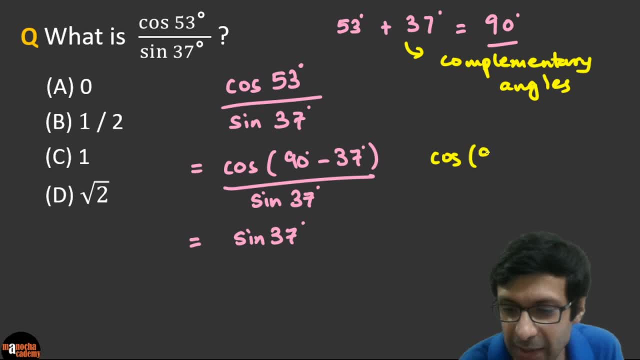 what is the formula we applied here? Cos 90 minus theta. Do you see that It's going to be equal to sin theta? That's the formula we've applied, right. So can you see cos 90 minus theta. That's the formula we've applied, right. So can you see cos 90 minus theta. That's the. 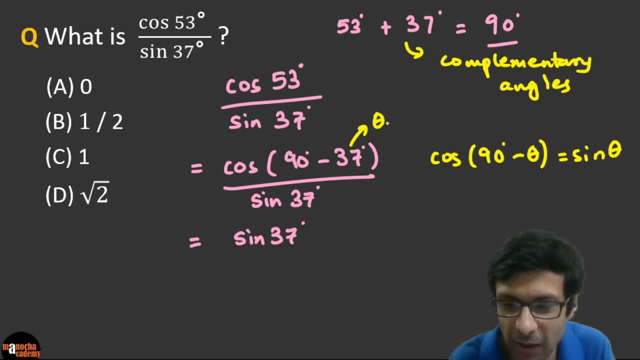 formula we've applied right. So this is our theta, Can you see? So it's going to be sin 37. And we have basically divided by sin 37. So the trick is we are changing cos into sin here in. 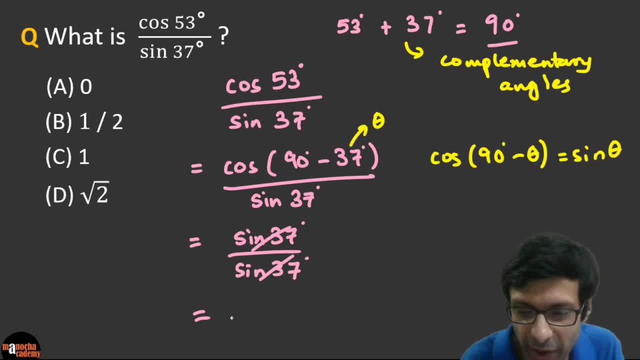 this step And you can see that these two are going to cancel. So very good guys, A lot of you got the correct answer. It's basically going to turn out to be: 1. Excellent, Superb, Clear. So that's how we apply our complementary angles. Now, guys, can you solve this? 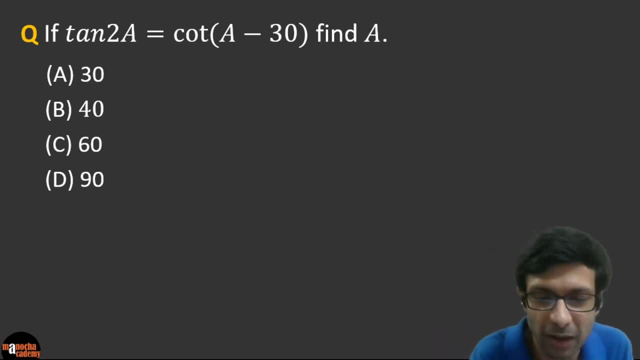 question for me. If tan 2a right is equal to cot of a minus 30, you need to find a. So come on, guys. I want all of you to try, And it's excellent to see everyone participating here. 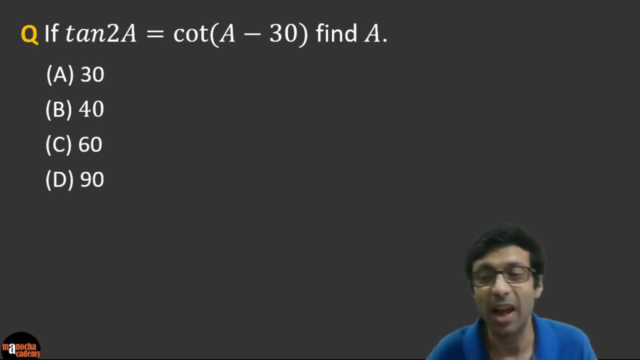 And, guys, if you haven't hit the like button, please hit it right now And do share out our videos with your friends so that we can have more people join the Manocha Academy family. So, guys, try out this question. So I have another this interesting question for you. 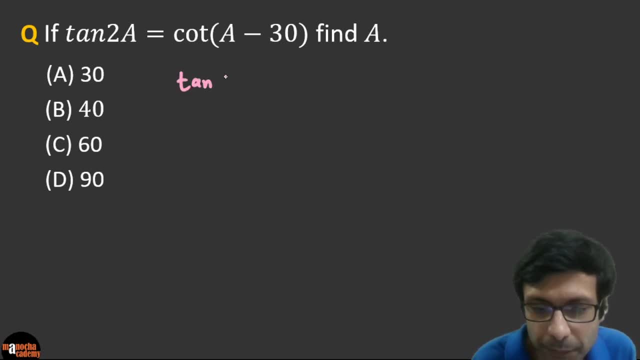 which what do we have here? Tan of 2a, okay, is given equal to cot of. so we have. so let's write that in blue here. So cot of a minus 30. And we need to find a. So the question: 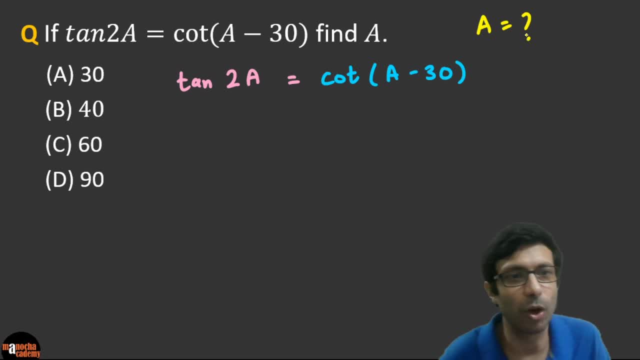 is we need to find a here right. So come on, guys. Excellent, I see some answers already. Superb, I want all of you to try this Right. So what do we do here? So what can we do? So we've got a tan on the left and a cot on. 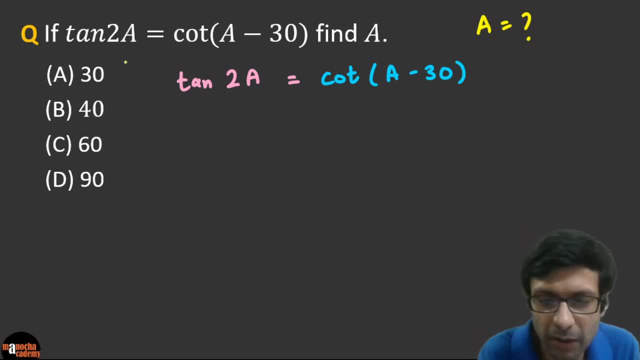 the right right. So we can't directly compare these guys right. So we can't compare 2a and a minus 30 because we've got tan on one side and cot on the other. So let's see if we can. 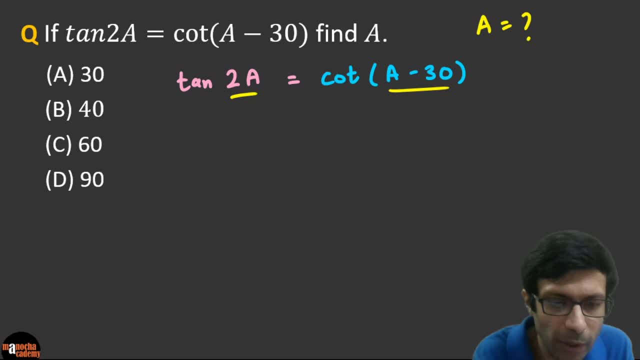 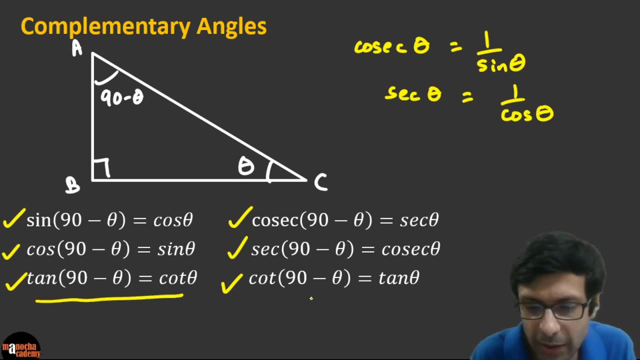 apply some of our concepts to convert right. So what is the formula we learned here? Let's take a look. So, guys, can you see this formula right? So we have tan 90 minus theta equals cot theta. 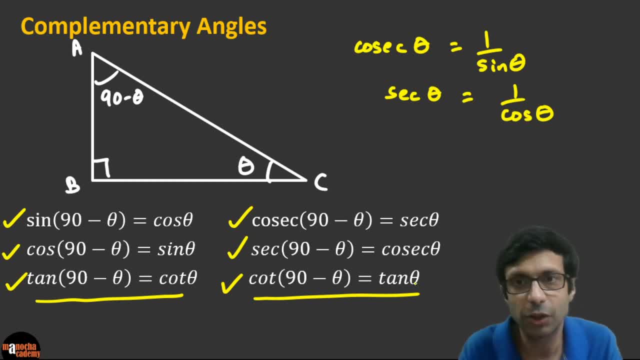 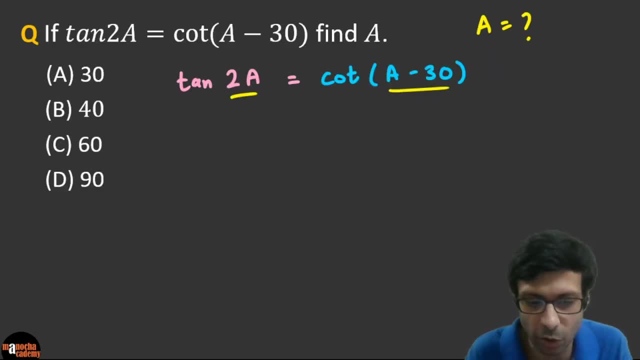 90 minus theta is tan theta. So I would suggest you to write down these formulas, right So, when you're solving the question. so either you can write it while solving or you can write it on the side, So whatever you feel comfortable, right? So what have we learned, That cot of? 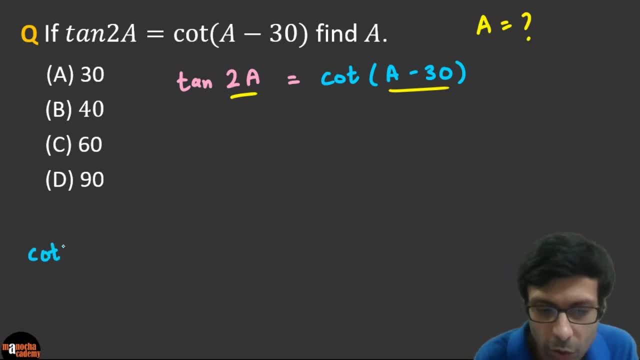 so we know. so let's write it on the side here. So cot of 90 minus theta is basically equal to tan theta right. And similarly we also know that tan of 90 minus theta is cot theta right guys. 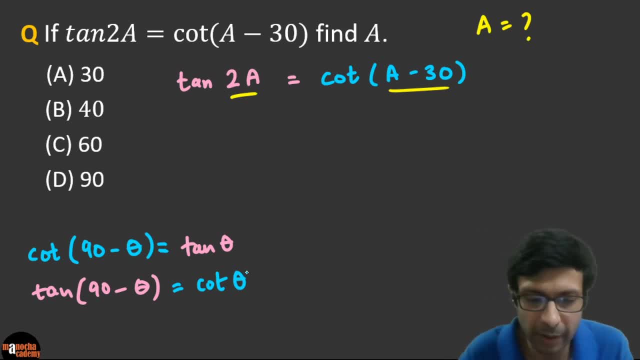 Okay, So we have that. So let's see which one we can apply here. So let's convert our left-hand side So we can convert the tan into a cot. okay, So let's try to do that. So that should be. 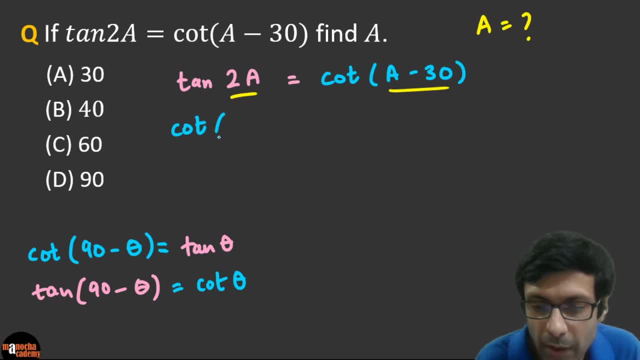 so the left-hand side will basically become cot of 90 minus 2a, right? Do you guys agree? Because tan 2a is going to be tan theta is cot of 90 minus theta, So can you see we are using this. 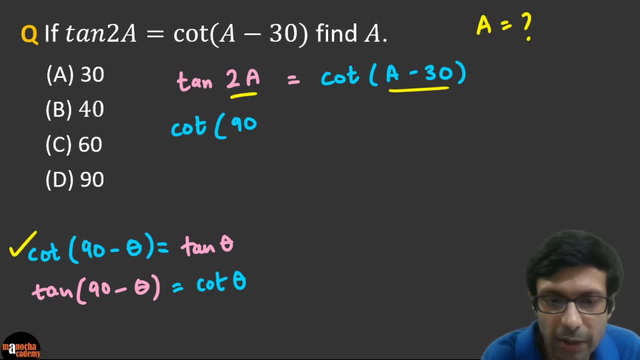 relation here. So let's convert it here. So it's going to be tan 2a is going to be cot of 90 minus 2a, and that's equal to cot of a minus 30.. So does everybody follow me? Very good, I'm seeing. 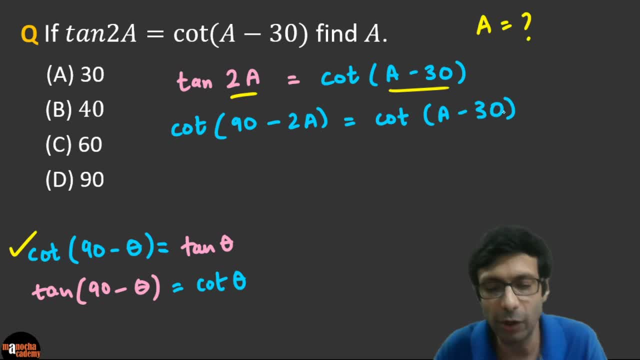 already some answers here. So see what's the trick. We are converting tan to cot. Why So that now we can compare? because we have cot on the left and right. So therefore we can say: these angles are these things in the cot, the angles are equal. So 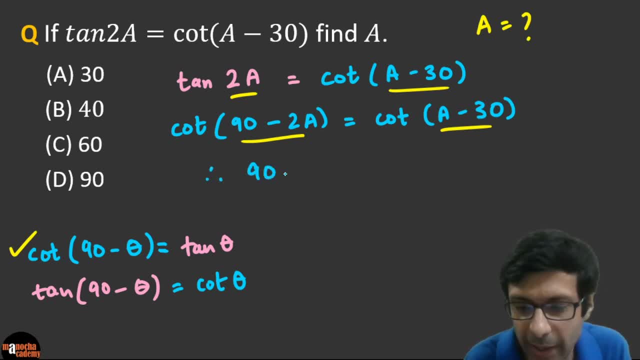 therefore we can write here: So therefore we can say: 90 minus 2a is equal to a minus 30.. We can equate it now, right, And so now, if you solve, we can get 90 plus 30 we'll get is equal to 3a. 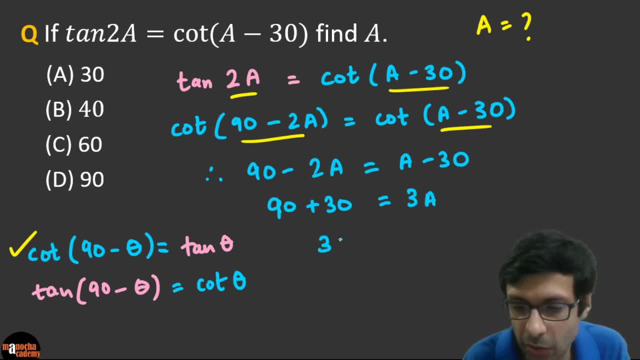 goes on this side. So therefore, what am I getting here? So let's reverse it and write: So we have 90 minus 2a is equal to a minus 30. So what is the answer, guys? What are you guys getting? Excellent, I see a lot of people have got the correct answer: 120 by 3, 40 degrees, Superb. That's absolutely the right answer. Now you may be asking: can I convert the right hand side cot to tan? Of course you can do whichever one right, So we can do that also. So suppose you want to convert this guy. So this guy will become basically tan of 90 minus. But we need to be a little careful here. Let me write it again clearly. 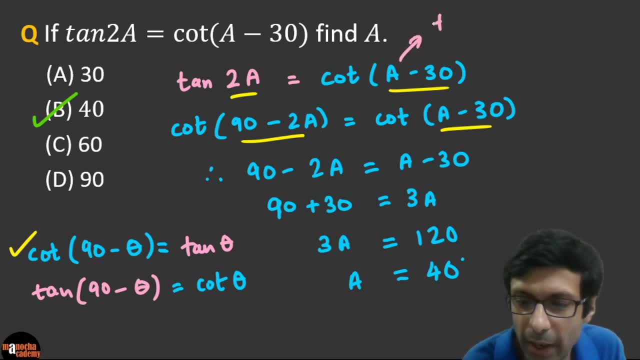 So, guys, if you want to convert this cot guy, So we'll have to write tan of 90 minus a minus 30.. Be careful, You need to put that angle in the bracket, So then it will basically become tan of 90 minus a plus 30.. Okay, guys, And so you're going to get something like tan of 120 minus a right. So again, if you solve that and equate it, you're going to end up with this. 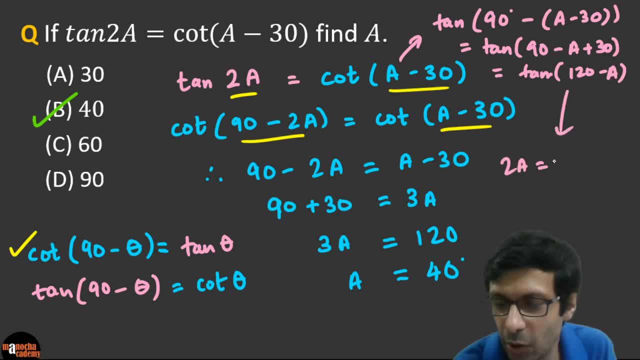 So 2a equals. So you can see from here, 2a equals 120 minus a. Therefore, 3a is 120. And again we are getting, a is 40 degree. So, whichever way you go, And, guys, you can see that this the one on the left- the first option worked out faster because we didn't have to deal with that big angle, But both way you get the same answer. Excellent, guys, Superb. Okay, So we are using complementary angles. right Now I have another interesting question for you. 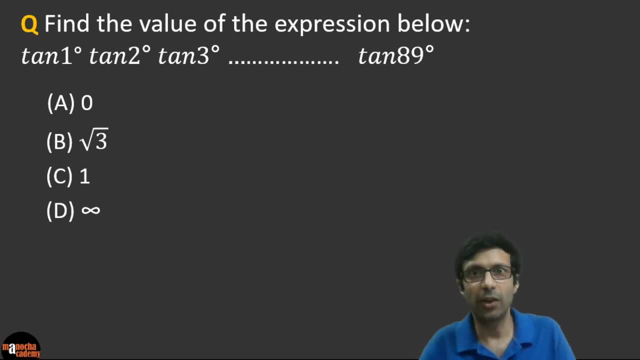 Okay, So let's put this expression below: Tan 1 degree, tan 2 degree, tan 3,, tan 4, and so on all the way up to tan 89. So you're multiplying these, right? So tan 1 multiplied by tan 2, multiplied by tan 3, all the way up to tan 89.. So, guys, what do you think this is going to be? Wow, I already see some answers. Excellent, guys, Excellent, Very good, You guys are trying. So let's see how can we solve this interesting, long question. 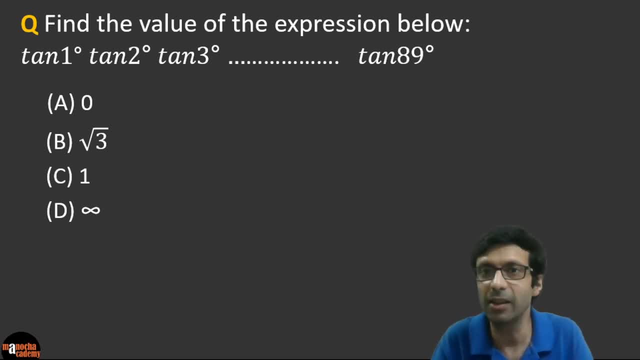 Okay, So let's see how can we solve this interesting long question, Right? Because there are, I think, 89 terms here, right From 1 to 89.. Wow, that's going to be a lot of terms. So let's see how we can attack this question, right? So let's take a look. So let's write it down first. So what do we have here? Tan 1 degree right Multiplied by. so we are multiplying this times tan 2 degree, multiplied by tan 3 degree right, And so we have a lot of terms here, Right? So let's take a look. So let's write it down first. So what do we have here? Tan 1 degree right, Multiplied by. so we are multiplying this times tan 2 degree, multiplied by tan 3 degree right, And so we have a lot of terms here, Right? So let's take a look. So let's take a look. So let's write it down first. So what do? 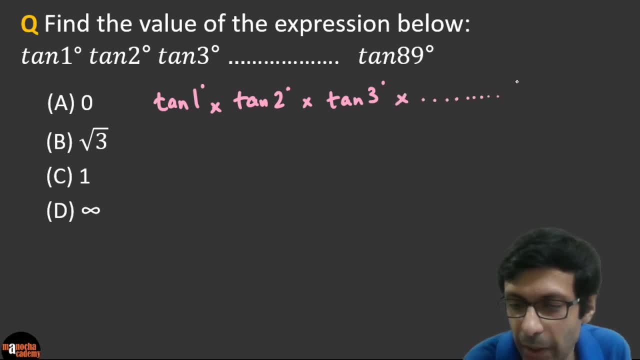 angles here. so- and it's the question, i'm just copying it down right now. so it's all the way up to tan 89, right? so what are the things involved here? let's rewrite it clearly. so we have tan 1 times tan 2, right, and so if i continue, it's basically going to be tan 44 here. 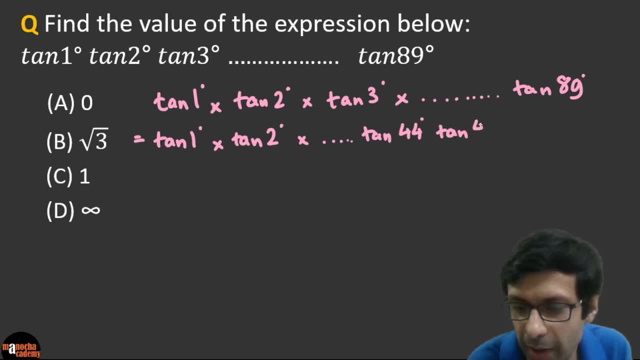 then in the center we have tan 45, right, guys, then tan 46, right, we continue. then we'll have tan 88, so i'm writing some more terms and tan 89, does everyone agree with that? so we're just basically multiplying out here, right? so now, what concept we can use here, guys, think about it. so what can? 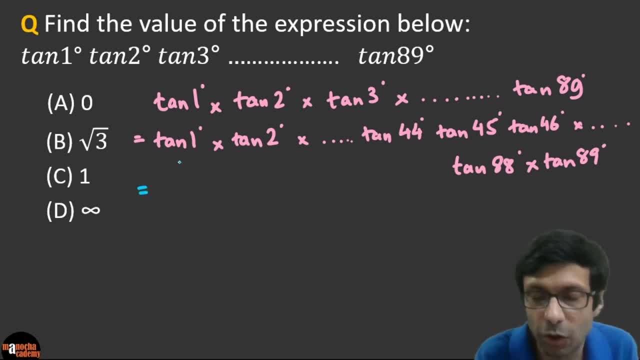 we do here. so can you see that this, using that relation right? you can see that this is the tan 45 right. so we have tan 45 right. so we're just basically that tan 90 minus theta is basically cot theta right, or cot 90 minus theta is tan theta right. 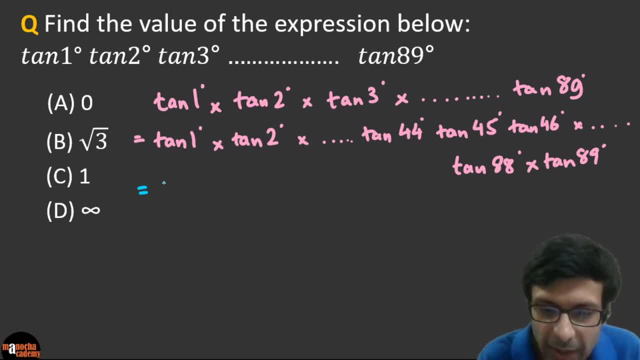 guys. so can i say that? so what can i say here? that tan 1 is basically going to be cot of 90 minus 89, right? oh, sorry, so this is going to be- let me write it again, my mistake. so tan 1 is basically going to. 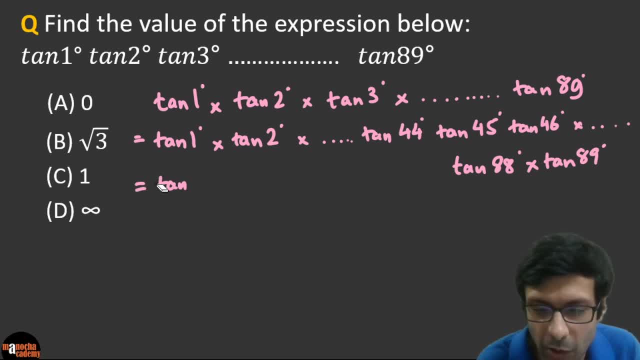 be let's right, so right. so write it a little lower so that it's clear to you. so tan 1 degree is going to be tan of 90 minus 89, okay times, tan of 90 minus 88, right? and this will continue. so then we'll get over here. 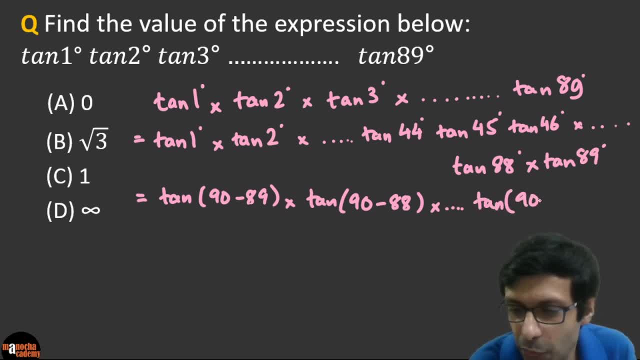 what do we get? tan of 90 minus 46 times tan of 45 and we continue. that multiplied by tan of this will reverse right, so this is tan of 46 here, so we won't do that. so tan of 46 and tan of 88 and tan of 89. okay, so can you see what we've done? so the initial part before tan. 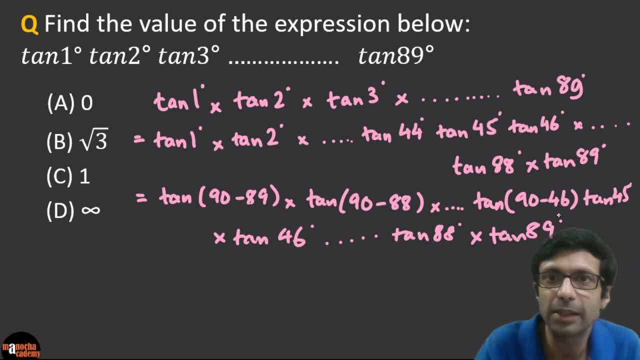 45, because 45 is the same tan of 88 and tan of 89. okay, so can you see what we've done? so the initial part before tan 45, center point here. before that we've changed the angle from one degree to, into this, 90 minus theta. 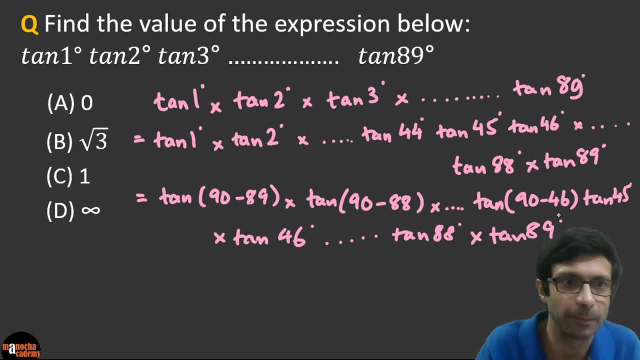 form right, because you know one is 90 minus 89, clear guys. so please take a look at the concept here. so now what we can use. so we are going to use the relation. so what are we going to use, guys? here can you see that tan 90 minus theta here. so we are going to apply the relation tan 90 minus. 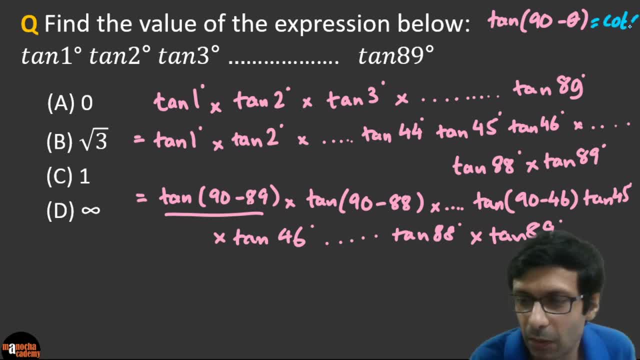 theta is basically cot theta. right, the thing that we're going to use is tan of 90 minus theta for these complementary angles. so tan 90 minus theta is cot theta. so what are we going to get here, guys? so the first term is basically going to be cot of 89. do you guys follow me? because it's? 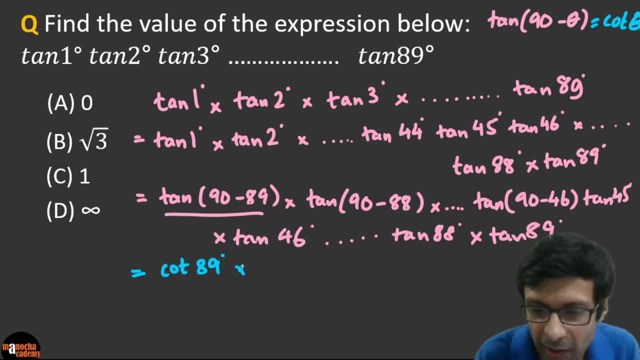 tan 90 minus 89, which means it's cot of 89 degree. the second term is basically going to be cot of 88 degrees right, and so on. it will continue. and then we have basically cot of right, so we have cot of 46 degree here, right. tan 90 minus theta is cot of 88 degrees right, and so on, it will continue. 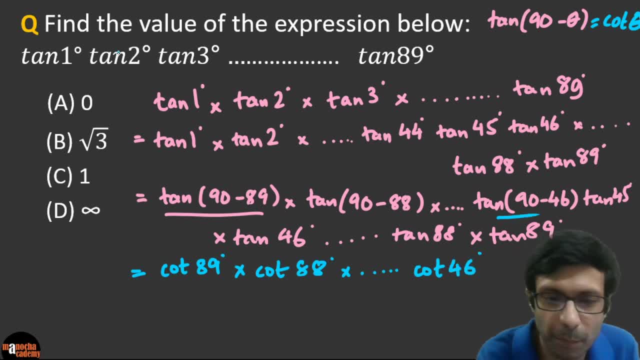 and so on. it will continue. and then we have basically cot of 88 degrees, right, and so on, it will continue. 46, can you see? this term changes to cot of 46 and multiplied by these terms, we didn't change. so we have tan of 45 right times, uh times, tan of 46. okay, i think you guys can't see that, my head. 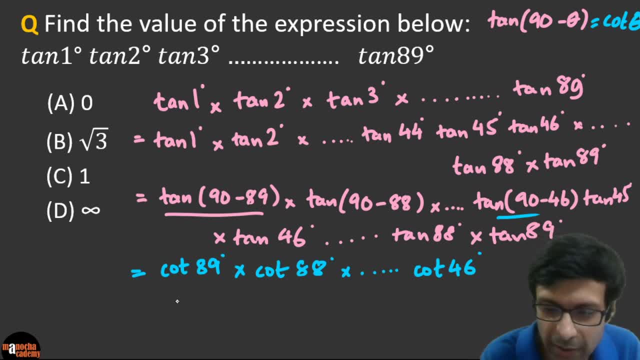 is covering, right, so let's write it clearly here. so we have this thing: times tan of 45 degree here, right? so times tan of 46 tan 88, times tan 89. so does everyone follow me? it's pretty simple. so all we've done is we are changing the. 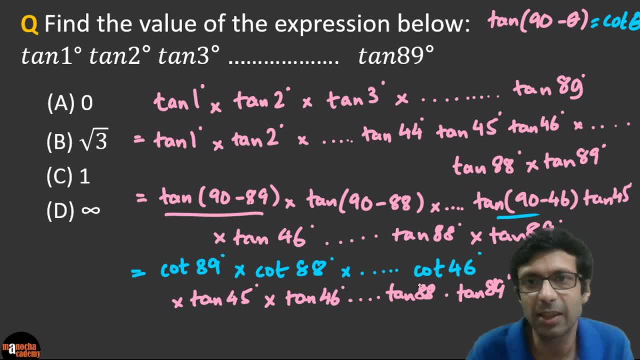 one degree to 90 minus 89. so tan 90 minus 89, cot 89, cot 88, and we go on till the center, because 45, you know, is the center thing. now comes the interesting thing: you know that cot 89 is 1 by tan of 89, right? so can you see, guys, this term and this term will cancel, because they are. 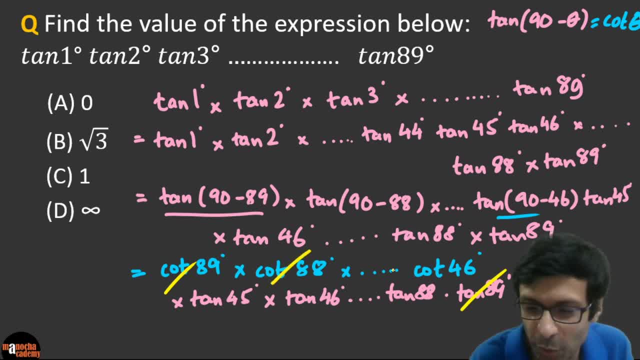 reciprocals. again, cot 88 and tan 88 are reciprocals. they will cancel each other, since we were multiplying them. similarly, cot 46 will cancel with tan 46. so finally, we, what are we left with? guys, only, we are left with tan of 45 degrees. right, so we are left only with tan of 45. 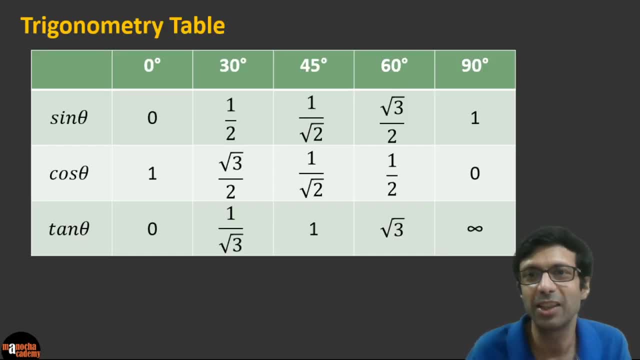 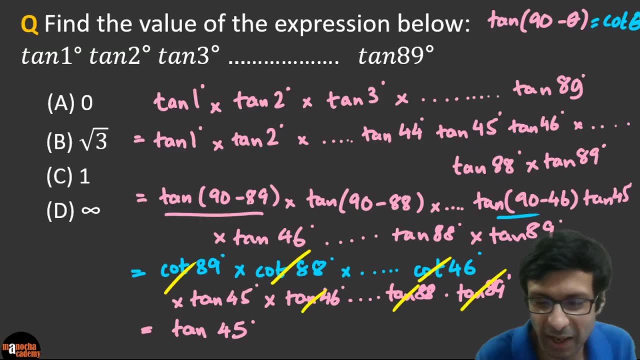 and guys, you know from the table what is tan of 45? it's one one, right? can you see the value here? tan of 45 is one, so very simple. this answer is going to be turn out to be one excellent, and lot of you got the correct answer. so it's one here. and so we, uh, changed this whole huge expression. 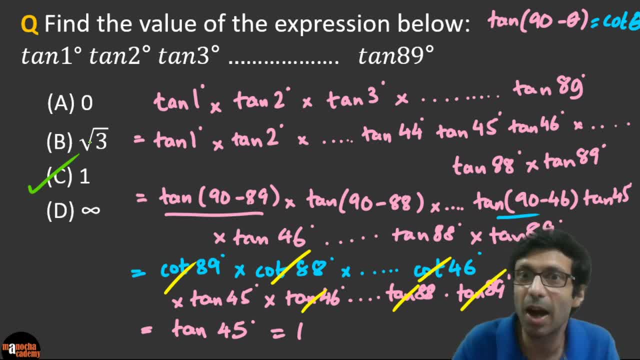 using the complementary angle formula tan 90 minus theta is cot theta right. so we changed the tan into a cot for half of the terms and we cancelled it, and so we got one superb. so, guys, that was an interesting question. i hope you guys got it. if you have some doubts, you can put it in the comments or 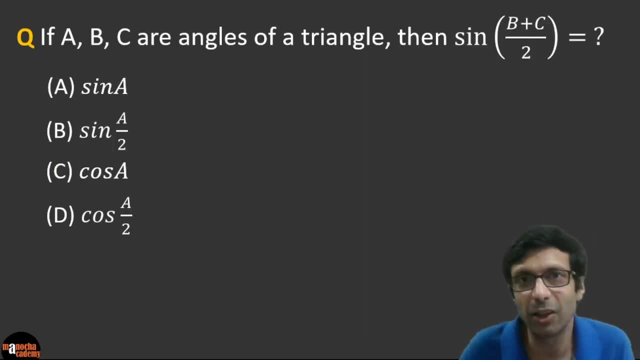 watch this uh video again. so let's move on to another interesting question. if a, b, c are angles of a triangle, then sine of b plus c by 2 is going to be what. so, guys, can you tell me? okay? so some of you asking: how do we know to convert? so, guys, you'll see the clue here, right? 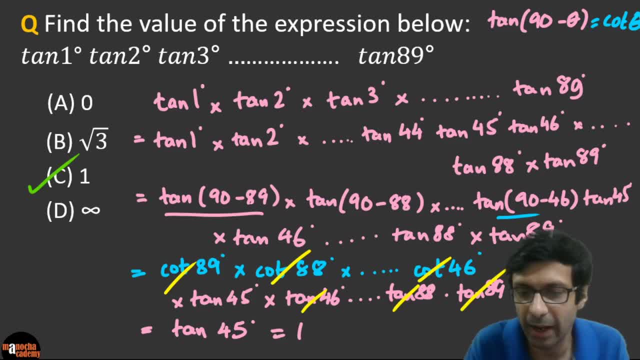 so did you see the clue here? because you had this: 1 and 89, so you have 90 minus 89. 2 and, uh, 88. they are complementary angles. so you have to look for these clues and then apply the formula okay, and you'll get this with practice, don't worry right, you just need to. 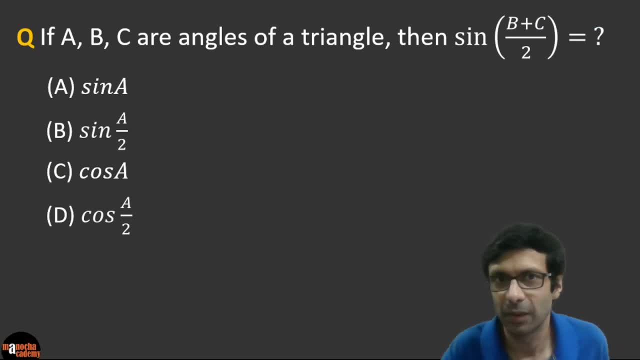 practice. so now please try this question, guys. so i want all of you to try. so come on, guys, try this question. if a and a, b, c are angles of a triangle, right so we've got this triangle here, so let's draw it down here. so let's say we have a, okay, right, so we have this: a, b, c. 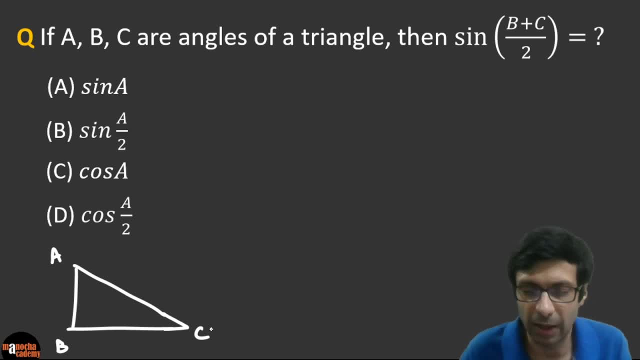 right. then sine of b plus c, right, and it should be basically a right angle triangle, right. so here, so we have a, b, c are the angles of a triangle. then we need to find sine of b plus c by 2, right, so we have basically a plus b. 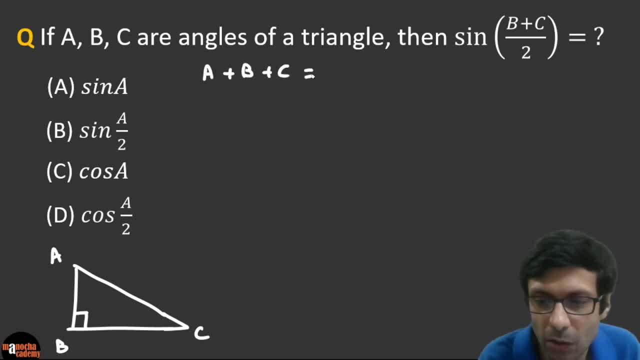 plus c is 180 degree here, right, guys? okay? so, uh, all of you know, right. so in the triangle we have angle a plus b plus c is 180. okay, so now what do we need to do? we need to find sine of- so let's write that down clearly here- sine of b plus c by 2.. so what is that going to be? 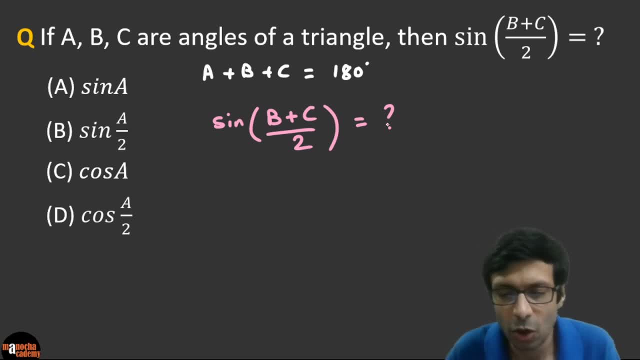 so, very good, i can see some answers here. excellent, you guys are trying. so what is the trick here? so let's apply what we know it's going to be: sine of. we know, uh, the angles are adding up because they they're angles of a triangle, right, so we'll get basically 180. so b plus c is basically going to. 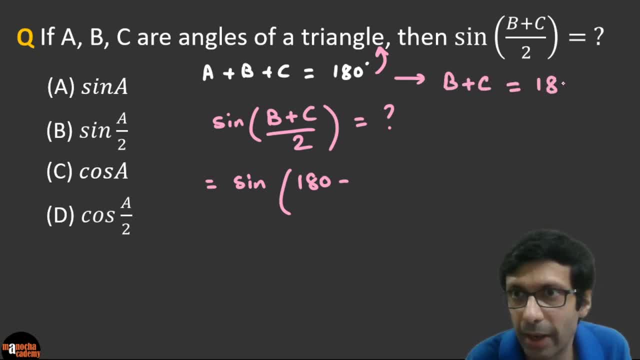 be. so let's write that down clearly: here b plus c is going to be 180 minus a, and let's substitute that here. so can you see, here we are substituting in b plus c. it's 180 minus a by 2, right? so let's. 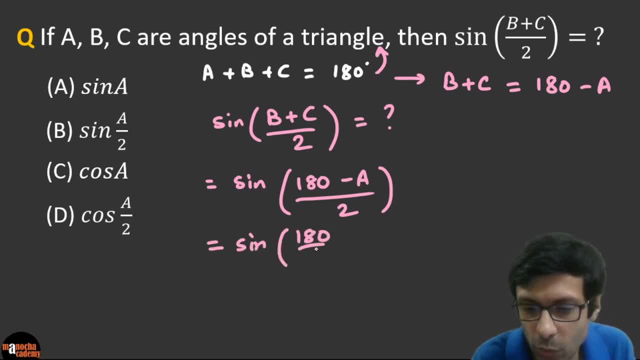 write that down. so that's basically going to be 180 by 2 minus a by 2, right, okay? so that's basically sine of 90 minus a by 2. so can you see that, guys? very good, so sine of 90 minus a by 2. 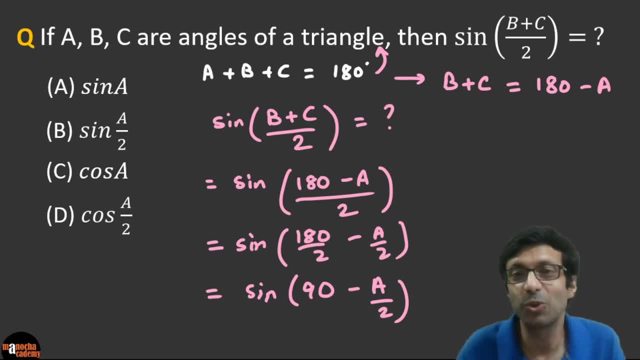 so what is that going to be, guys? so you know again, we can use sine: 90 minus theta is cos theta. so this is going to change to cos cos of a by 2. very good, very good, a lot of you got the correct answer. great guys, you guys are awesome, you guys rock. very good. you solved this question correctly. 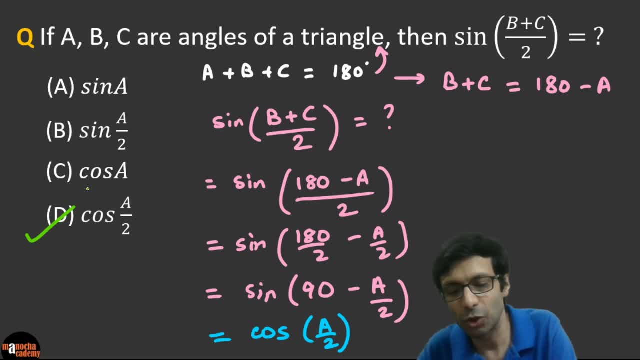 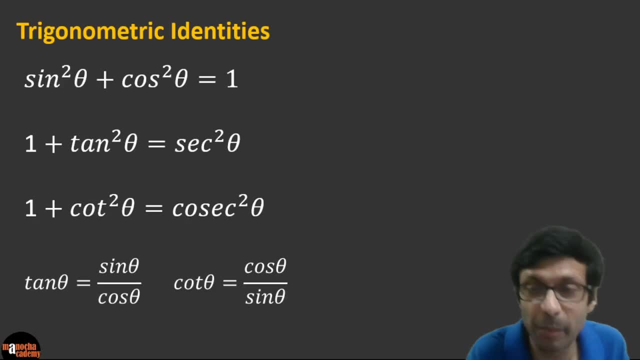 so very simple. you just substitute it and just make sure you do that 90 minus a by 2 correctly, and you have the right answer. excellent. so now we've done complementary angles, let's move on to trigonometric identities, right? so what are the identities that we have here? so these are these. 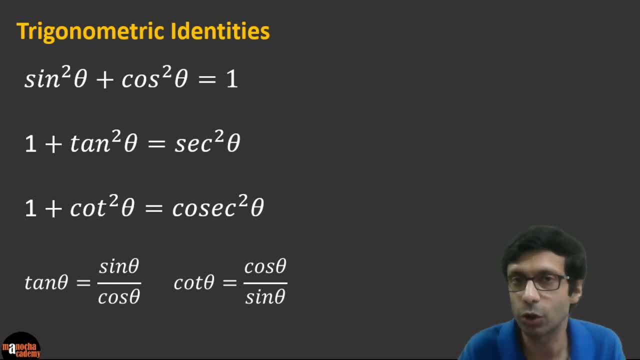 square relations, right where you have sine square theta plus cos square theta is 1, and then 1 plus tan theta is 1, and then sin square theta is 1, and then sin square theta is 1, and then sin square tan square theta is sec square theta. 1 plus cot square theta is cosec square theta, as 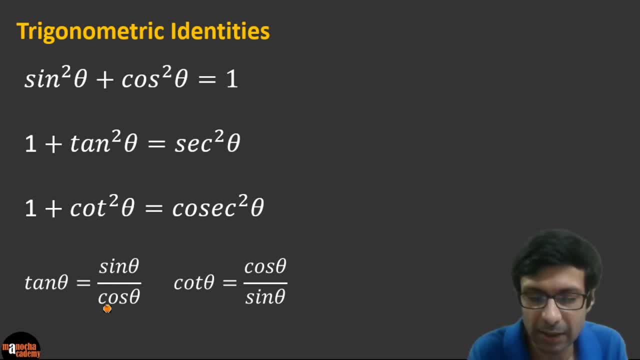 you can see here, and guys, you know that tan theta is basically sin theta by cos theta. I have just written this for your reference, useful to know. and cot theta is cos theta by sin theta. So let us try to understand what these guys are. So one thing, you guys. 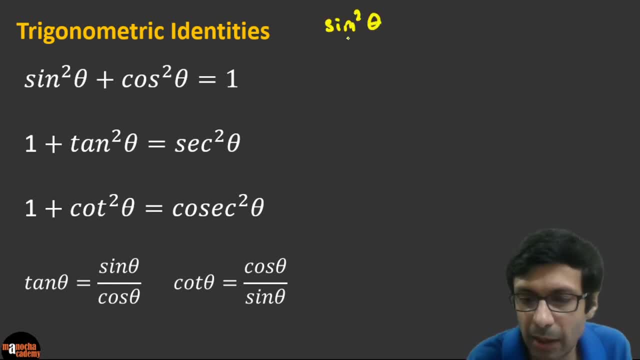 should know that sin square theta. what does it mean? it basically means- let me write that a bit clearly here. So when we say sin square theta, so we are basically talking about it basically means sin theta- whole square right. So let us understand. for a right angle triangle. 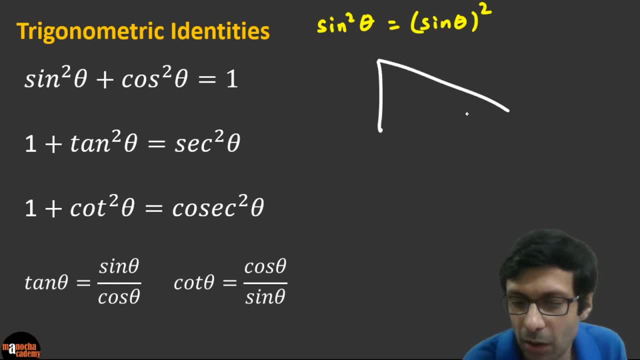 how do we get this relation? So it is pretty simple, guys. So take a look here. very, very simple. I am going to show you. So if you take a triangle, ABC, right angled at B, and this is the angle- theta- So let us mark the perpendicular for this theta is going to be. 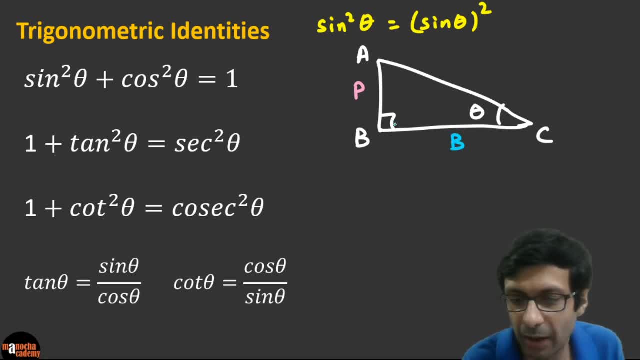 this side right. Base is going to be the right side right. So this is going to be this side right. So this is going to be this side right. So this is going to be this side right. So with the angle, theta and 90 and hypotenuse is opposite to the 90. So let us look at. 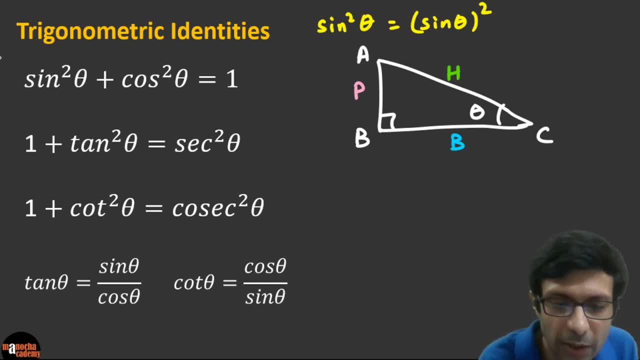 our first relation here. So, right, we are focusing on this relation, the relation 1, and let us see how we can easily prove it. So what is sin square theta going to be? So sin square theta is basically going to be. we said it is sin theta whole square. So 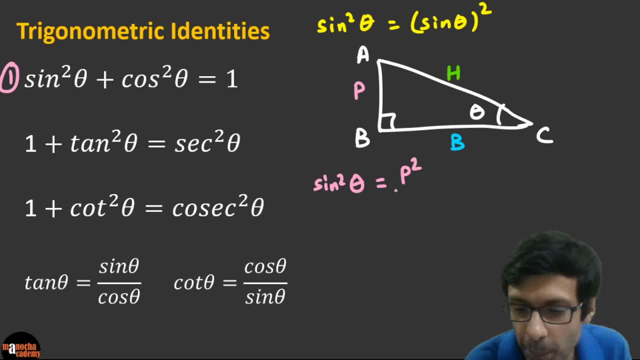 it is basically, you know, sin theta is perpendicular by hypotenuse. So P square by H square, right, and what is cos square theta going to be guys? So cos square theta is going to be sin square theta is going to be B square by H square, right, okay, B square by H square, and what is? 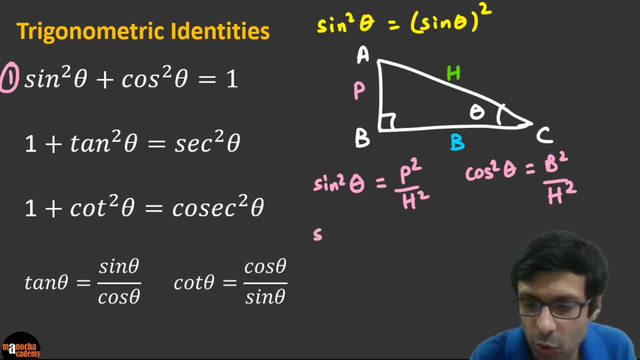 the first relation saying that add the two. So if we add sin square theta plus cos square theta, let us see what do we get. So sin square theta plus cos square theta is basically going to be P square by H square plus B square by H square. So what are we getting? So we 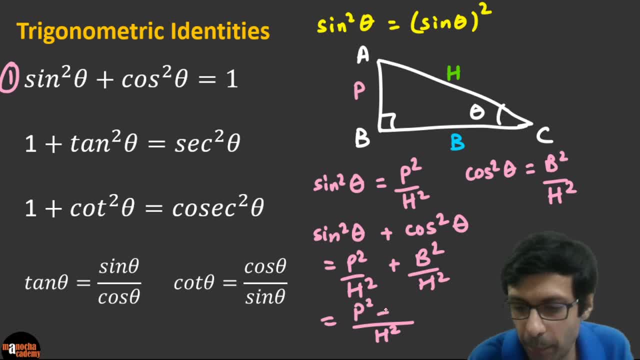 have H square in our denominator and cos square, theta is going to be B square by H square, P square plus B square, right perpendicular square plus B square. and guys, what is P square plus B square? okay, So what is P square plus B square? Is there an easy way to learn this? I am 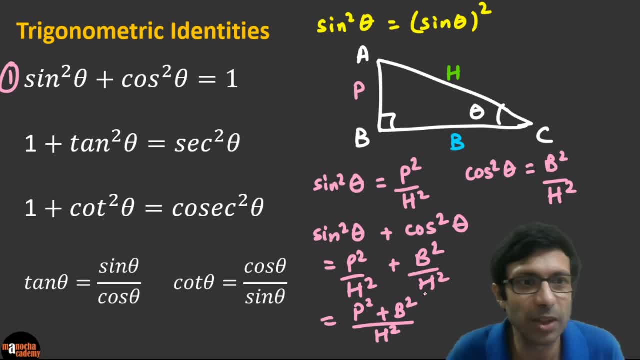 just going to show you, guys. somebody is asking, right, Drishti is asking: what is the easy way to learn? I am just going to show you how to remember these identities in a super easy way. So if you look at this by Pythagoras theorem, we know, guys, right, that H square is basically P square plus. 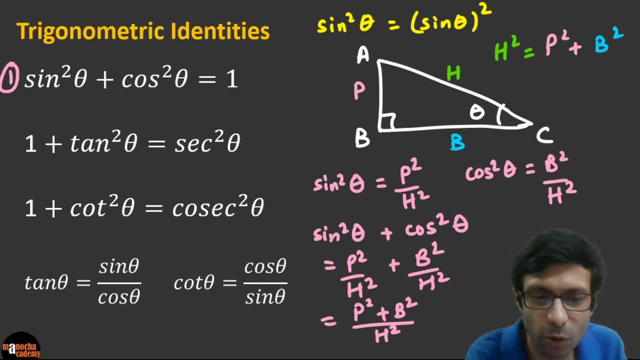 B square. you know from Pythagoras theorem. So this is basically going to turn out to be H square by H square, and that is why we get 1.. So can you see, guys, we have proved very simply sin square theta plus cos square theta. 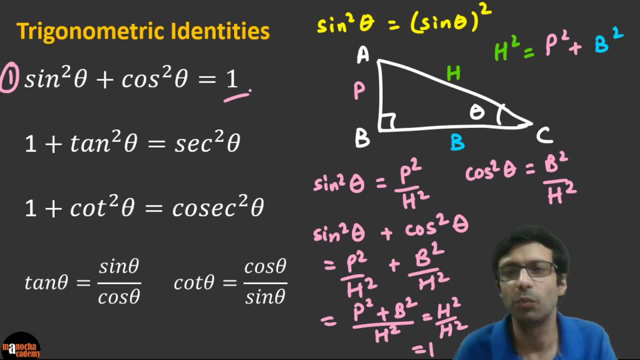 is equal to 1, clear. So if you look at this, we just substituted P by H and B by H and used Pythagoras theorem, as you can see here. Now let us see how can you remember and prove these, the second and the third identity? So let us take a look. So I am going to erase. 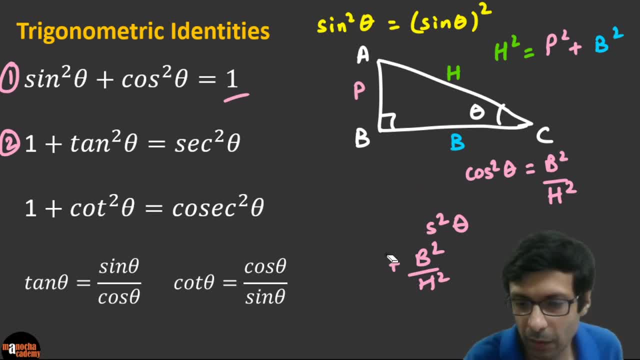 all of this, Since you guys have got it right, Okay, So let us just erase all this part here. So take a look, guys. how do you prove the second identity? in a very simple way. So come on, I want all of you to. 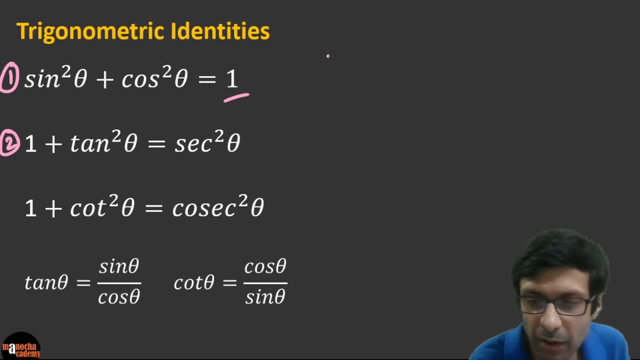 think here. So let us start with our first identity, since we have proved it. So let us write our first identity: sin square theta plus cos square theta is 1. right Now, to prove it, what do you do? You just divide it by cos square theta. okay, So let us just write it here. So let us just 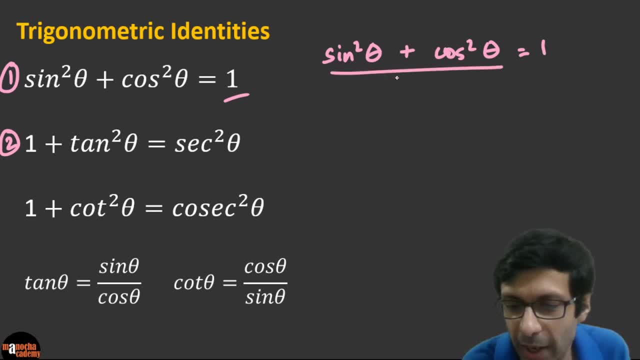 divide both the sides right. So we are going to divide this thing by cos square theta and the right hand side, left and right hand side. So what do we get? on the left side, Sin square theta by cos square theta plus cos square theta by cos square theta, right is equal to 1 by cos square. 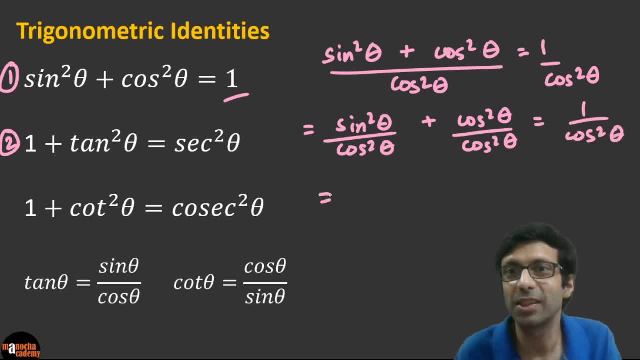 theta. Now, guys, see what are you going to get here. What is sin square theta by cos square theta? You can see, Can you see guys here? Sin theta by cos theta is tan theta. Look at this formula. So sin square theta plus cos square theta, this is going to be nothing but tan square theta, right? 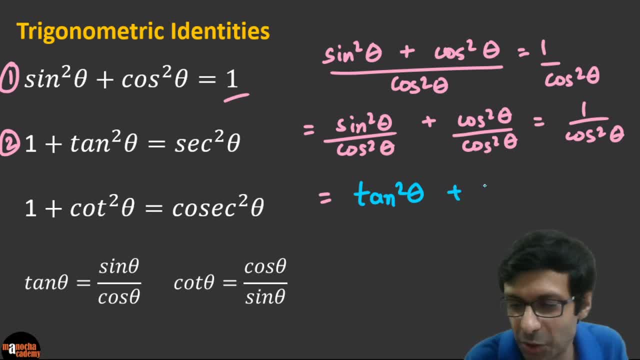 and this term cos square plus. this term is simple. This will cancel. It is 1. and what is 1 by cos square theta? You know that reciprocal of cos is sec theta, right? So it is going to be sec square theta, okay. So, guys, can you see that we have proved the second relation here: 1 plus tan square. 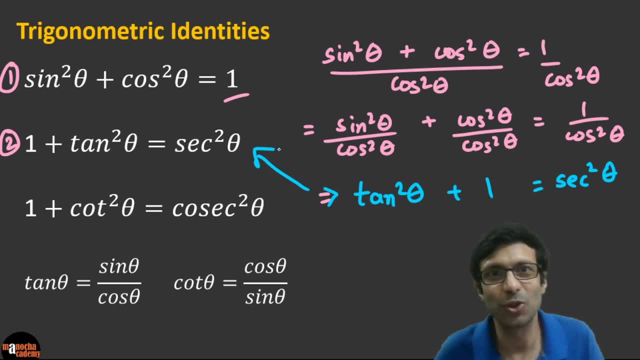 theta is sec square theta, okay. So, so simple, guys. take a look. We have simply proved it just by dividing by cos: square theta, clear and similarly, guys, you can prove the next one also. So I want all of you to try that. It will be pretty simple. You just need. 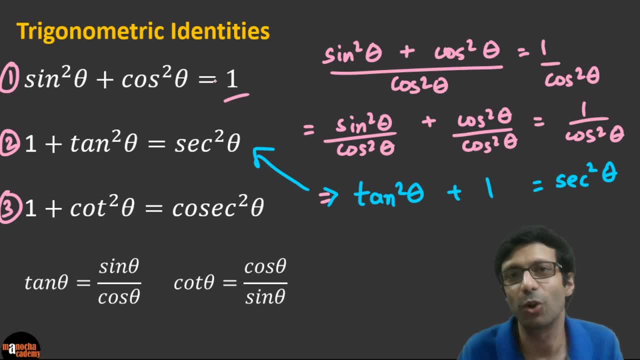 to divide the first relation by sin square theta. So you are going to get 1 plus cot square theta is cosec square theta. So you just need to remember that first relation and then the other ones are quite easy to prove. So once you prove it once or twice, you will absorb it and you won't. 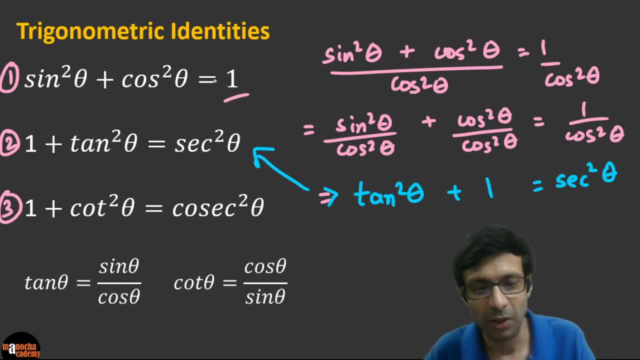 forget this. okay, Right? So just to summarize, some of you have a doubt. look at the first one. we proved it by Pythagoras, or you can watch the video again: sin square theta plus cos square theta was 1. and then what did we do to prove the second? Look at the proof of the second one. here We started with the. 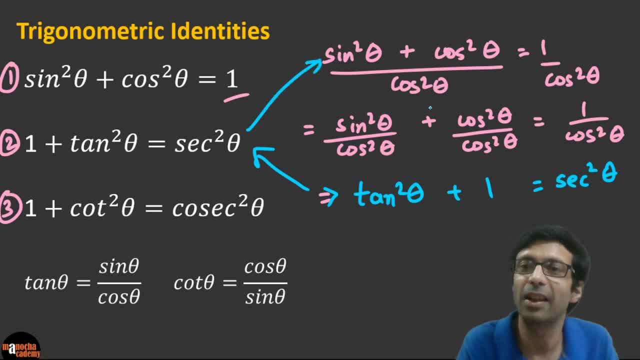 first relation right. and then we simply divided the left and right hand side by cos square theta, simple. Once you divide it, you will see that sin square theta by cos square theta is tan square theta plus 1 is equal to the reciprocal of cos square theta. So you can watch the video again. 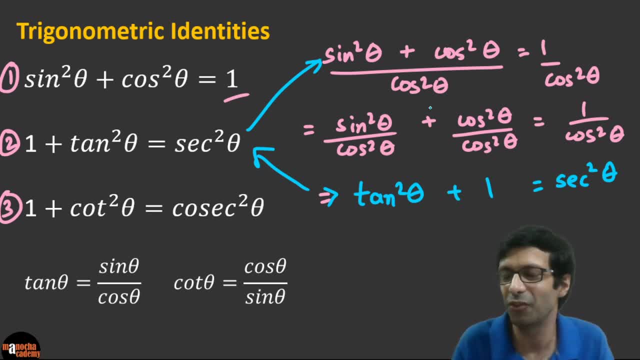 reciprocal of cos is sec square theta. So many formulas you have to learn in trigonometry, but after that it's really easy. and same thing for the last one. If you divide that first relation, if you divide it by sin theta right, So that first term, sin square theta by sin square theta. 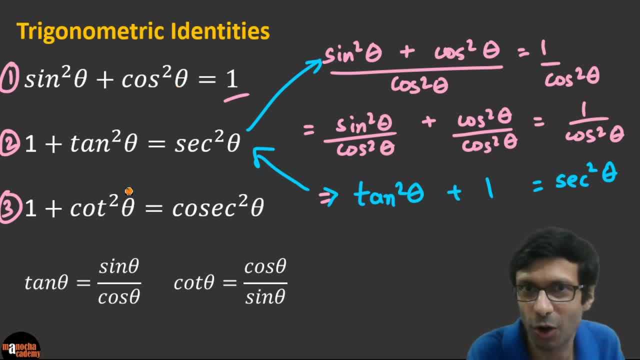 is going to be: 1 cos square theta by sin square theta is going to be cot square theta, and 1 by sin square theta is going to be cosec square theta. okay, and don't forget these important relations, also that tan theta is sin theta by cos theta and cot theta is sin theta by cos theta, So you can. 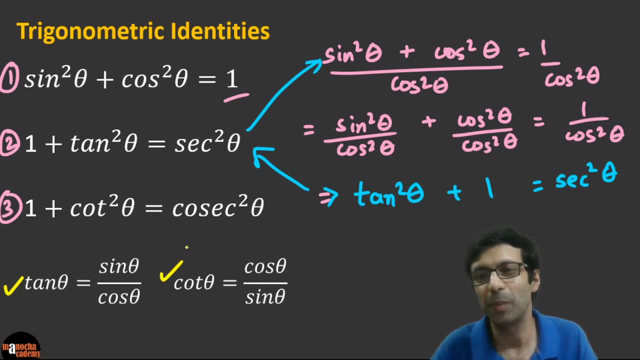 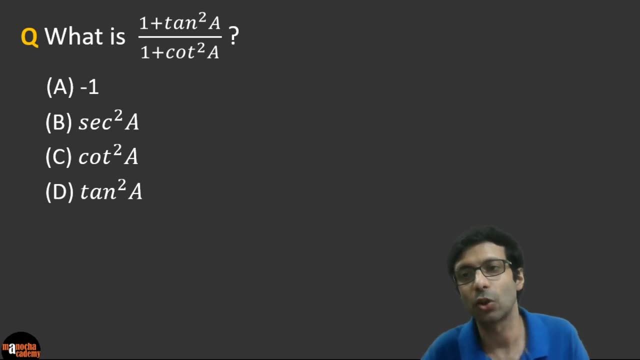 easily prove this. by p by h, b by h, the hypotenuse gets cancelled. okay, very, very simple. All right, guys. so to absorb these identities, are you ready to practice some questions? Let's try this. What is 1 plus tan square a by 1 plus cot square a, right Somebody had asked in today's class. can? 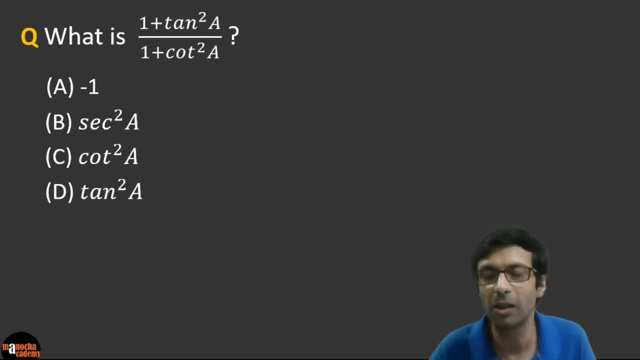 we use a also, yes, a, theta x, whatever right, these are just representing the variables, representing the angle, okay. So, guys, if you have any questions, you can ask me in the comments section below. Guys, please try this question. okay, I have some video requests for chemistry also. guys, we are 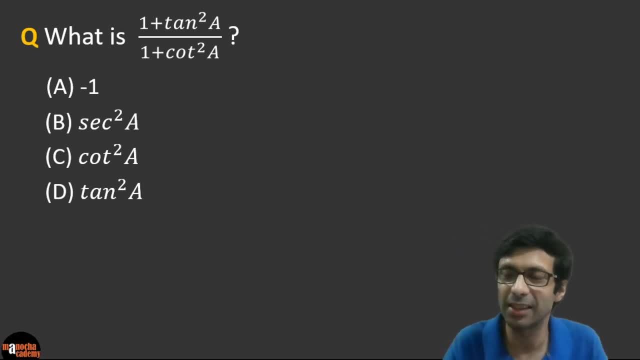 having during this lockdown. we are having daily live classes at 8 pm for physics, chemistry and maths, and we also have special live classes on our website, manochacademycom, So do check out our courses. they are at a huge discounts because we want to help all of you guys, So please do. 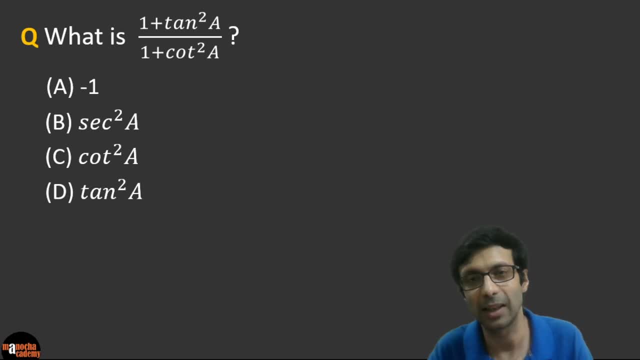 check it out. it's manochacademycom, we have the physics and chemistry course, and very soon we are going to be launching the maths course also. So do check it out and do share it with your friends. so, guys, try this question: what do you? 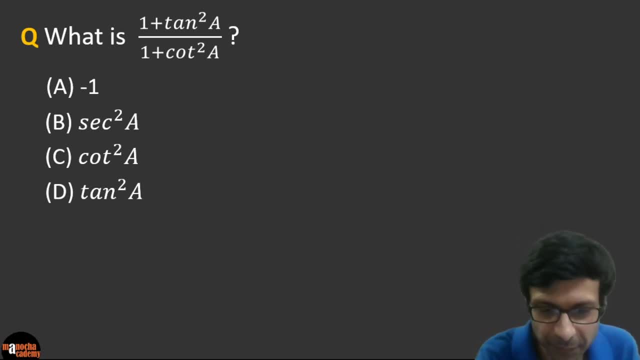 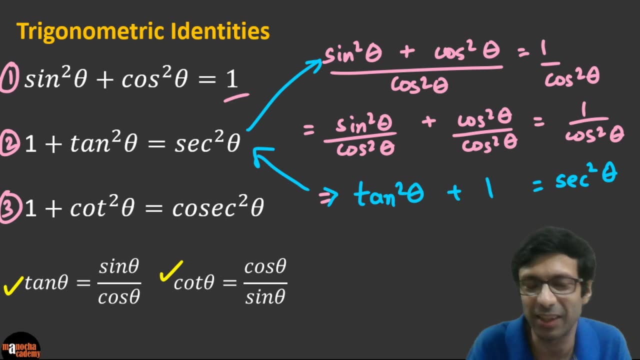 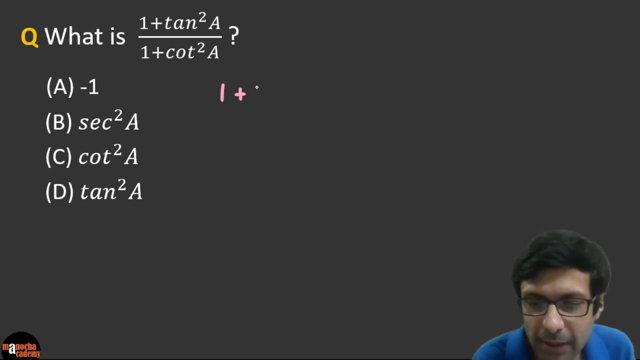 think this is going to be. come on, I want all of you to try it. okay, and hint guys, use these trigonometric identities that we've learnt. okay, so I've given you the hint. come on, let's try this question. what is the question asking? what is 1 plus tan, square a and trigonometry? 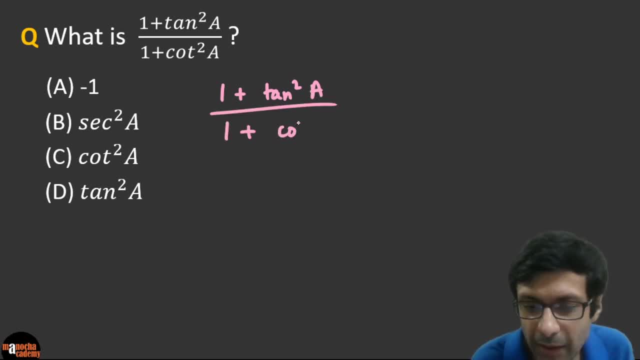 you just have to write down stuff, you know, write down the formulas on the side and work out the things right. so I would advise you, you know, write down the identities on the side. so let's write them down here quickly. so sine square theta plus cos square theta is 1. we learned that. 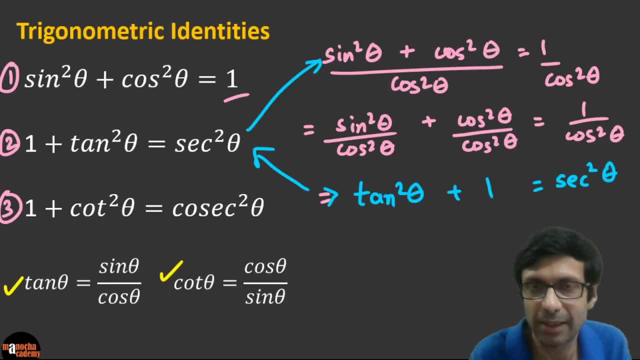 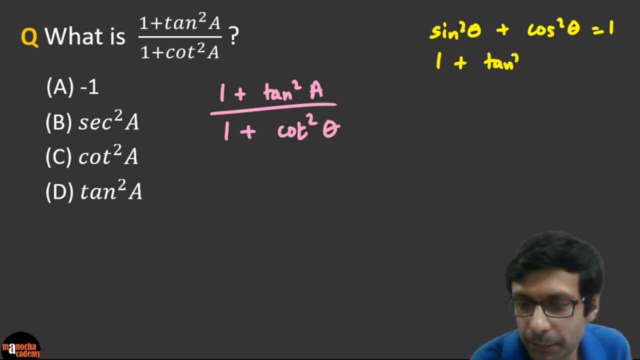 right. and what are the other identities? we saw: 1 plus tan square theta- right is sec square theta, right, guys? so we have: 1 plus tan square theta is sec square theta, and similarly, 1 plus cot square theta is cosec square theta. Okay, so write them in front of you so that you can see that. now let's see which of these. 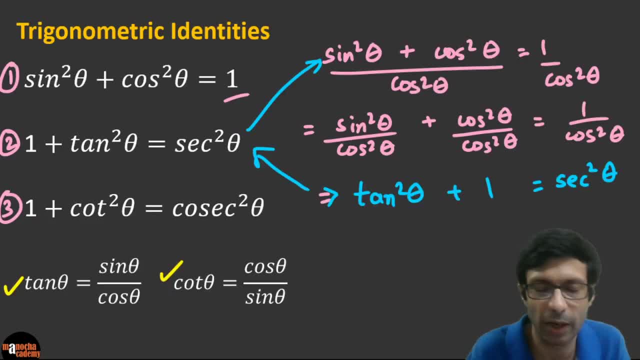 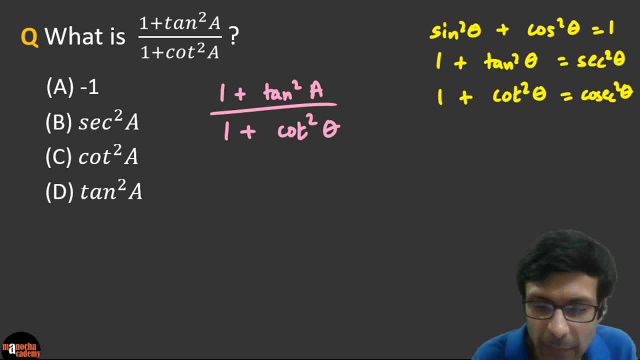 identities. so I just wrote down these three identities here, right, that we had learnt. okay, guys, simple, so please learn them and write them down, and that will really help you while solving the question, because you have them in front of you, so can you see from the identities? 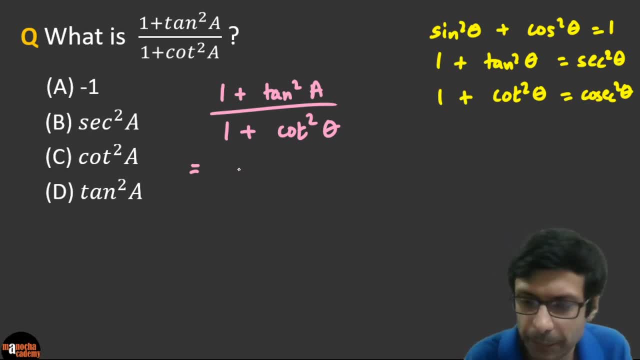 1 plus tan square a. what is it going to be okay. sec square a: right. look, we've used this identity and what is it going to be? What is it going to be Okay? sec square a is 1 plus cot square. oh, sorry, I wrote theta here by mistake. it should be a. my mistake, sorry guys. 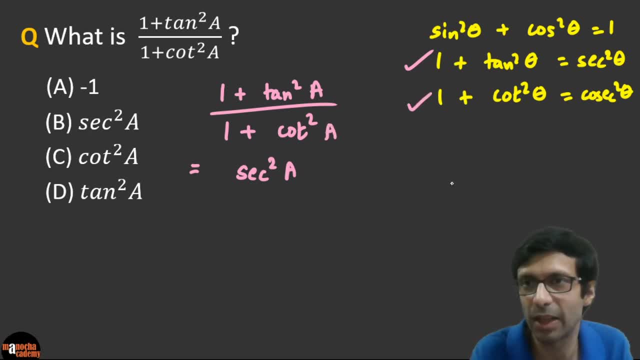 so what is 1 plus cot square a? it's going to be basically cosec square a, right, because 1 plus cot square theta is cosec square theta, so that's going to be cosec square a. okay, right, so that's what we have here. so now let's work out sec square a. you know, is basically the, the numerators, the. 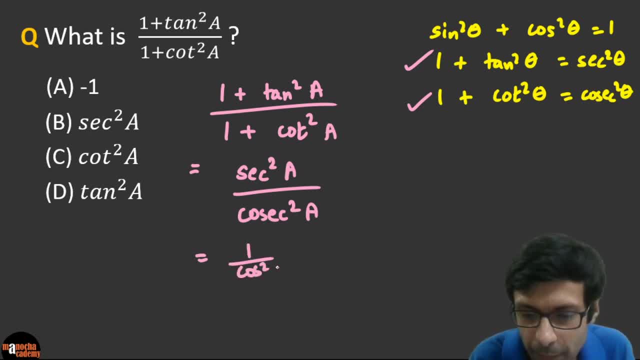 reciprocal. so it's basically 1 by cos square a and that's divided by. so the denominator is basically 1 by sine square a right, because cosec is the reciprocal of sine. so what do we have here, guys? so this is because we are doing division, so it's basically going to be inverted here. so 1 by 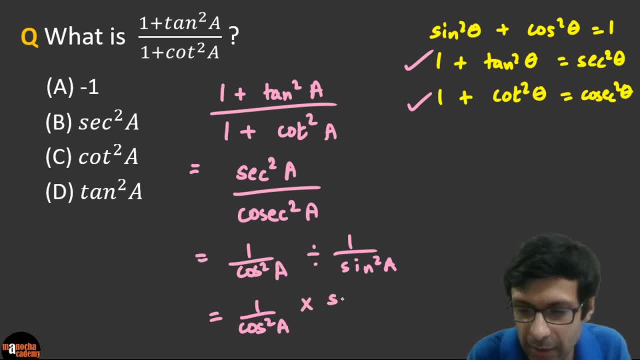 cos square a times. so this guy is going to get inverted sine square a, right you guys follow, pretty simple, and so let's see what do we get in the end. so we are basically getting sine square a by cos square a. very good, very good lot of you got it. 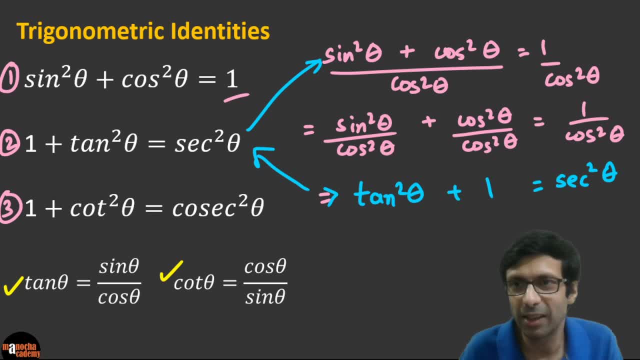 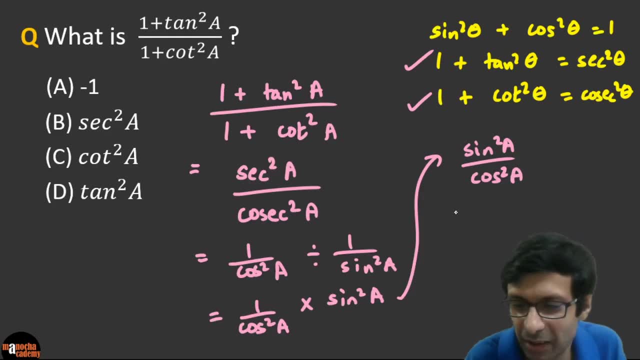 and guys remember this relation. what is sine theta by cos theta or sine a by cosec? can you see, guys, it's basically tan theta, right? so we are basically having here this is going to be tan square a. so did I do it correctly? please check it. very good, d is the correct answer. excellent. when will the? 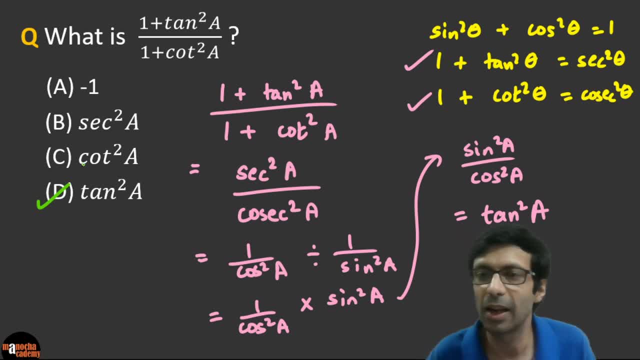 light class. be there tomorrow, right, it will be at. we have the class at 8 pm, right? so you can check the notifications. it's usually out around 5, 30 or 6 o'clock, right? so guys do join us for the live classes and this is the correct answer here. 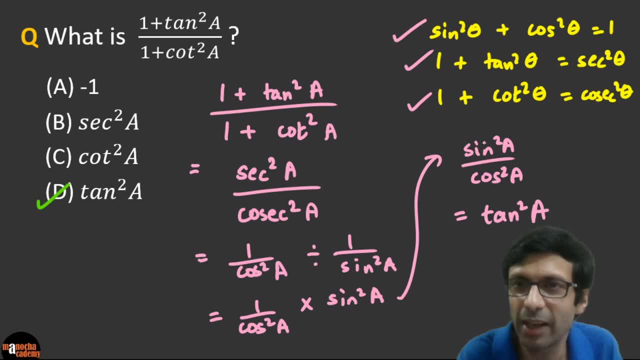 okay. so what was my main tip for you guys? please write down these identities. don't do it mentally right, because in the head if you're doing sine square theta, cos square theta, you're going to get confused. so write them down. it's not a waste of time, just write them quickly and just apply them. 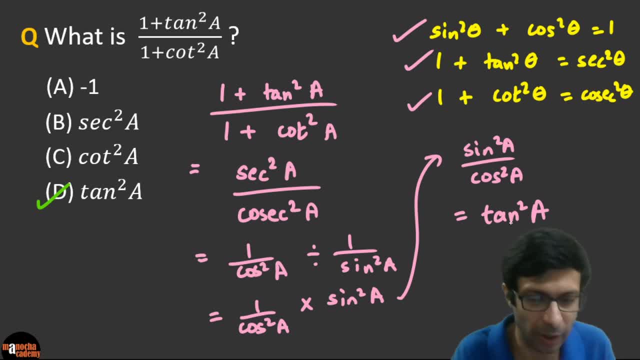 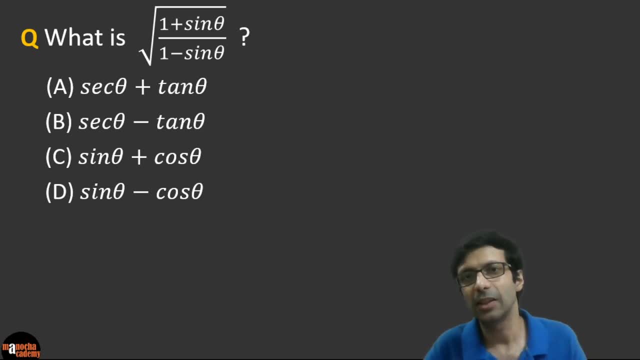 and you can see the question is really, really simple. okay, excellent, let's try this next question: what is square root of 1 plus sine theta divided by 1 minus sine theta? in trigonometry is all about simplifying the expression, looking at the goal you know and using your formulas and identities. okay, so, guys, please try it and guys do hit the. 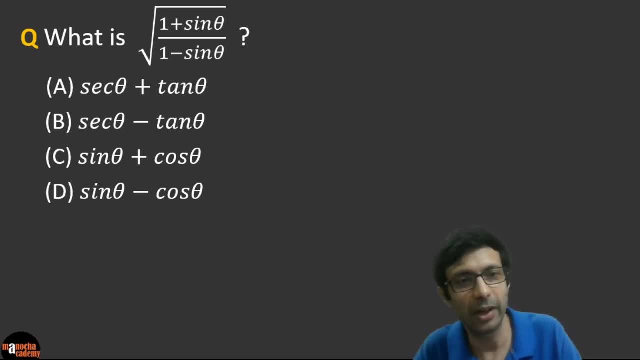 like button. I hope you're enjoying this session. you have been really interactive. I'm really enjoying it, so please hit the like button and share it with your friends. so come on, guys, try this question. so I hope you have your pen and paper ready, so always keep them for these. 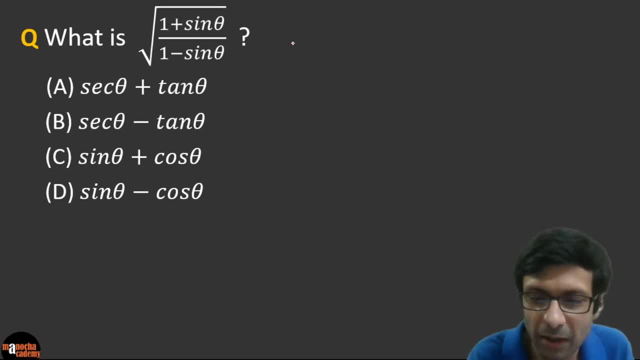 live classes so that you are totally participating in it, right? so I want all of you to try here. so the question is: square root of 1 plus sine theta, right divided by 1 minus sine theta. come on, guys. so what is this going to be? okay, very good. I'm seeing some of you are thinking of some. 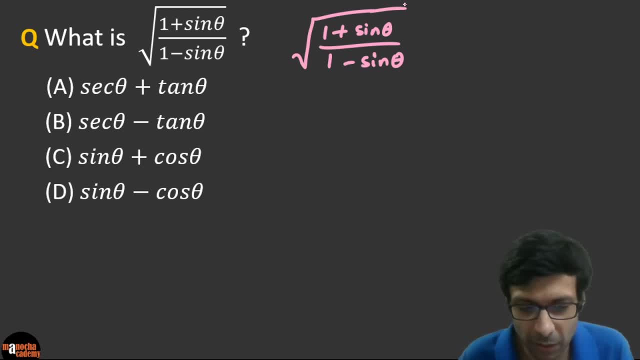 interesting things to do here. good guys, try it out, okay. so let's see what. what can we do here? so I want all of you to try this. so let's see that if we multiply the numerator and denominator, because we have 1 plus sine theta divided by 1 minus sine theta and we have this irritating square root, right. so let's try. 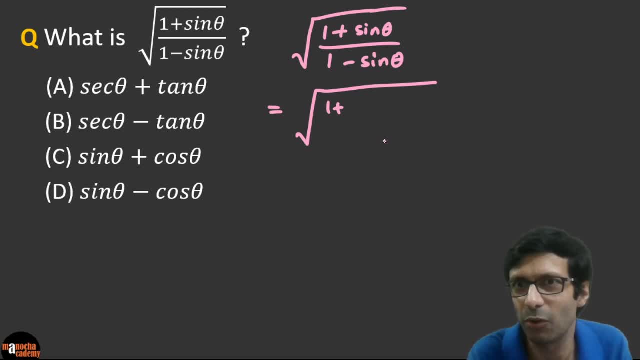 to get some square relation so that we can get rid of the square root right? okay, so let's see we can do so. let's say we take 1 plus sine theta and multiply that in the numerator right and in the denominator so that we don't make any change. so we are multiplying, can you? 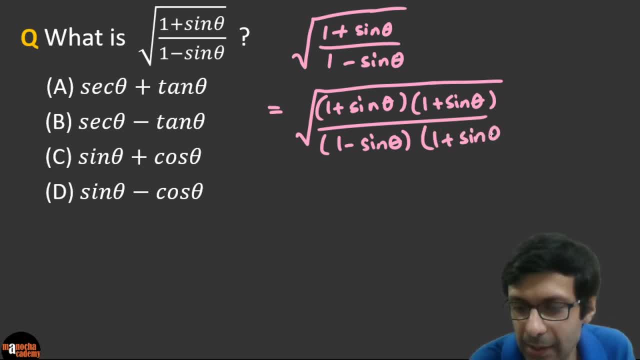 see the numerator and denominator by 1 plus sine theta. here we are multiplying the numerator and denominator by 1 plus sine theta. so what are we going to get here, guys? so we are going to get basically square root of. so this numerator is going to be 1 plus sine theta, whole square. 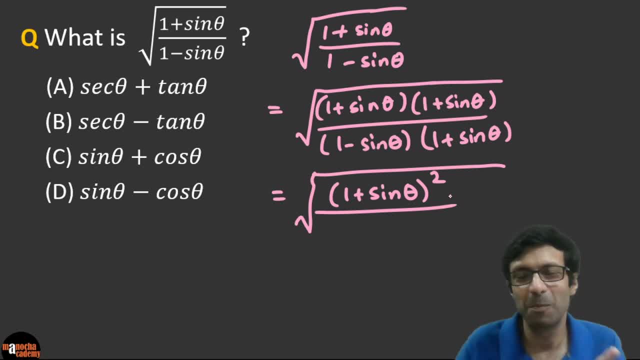 and what is this going to be? can you see, guys, a minus b multiplied by a plus b. can you see that? so we can apply the formula, guys, you know this relation right: a minus a plus b times a minus b is basically a square minus b square. so let's apply it here. and what are we going to get? 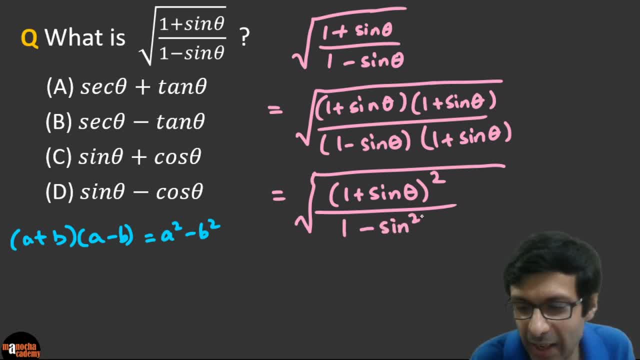 1: 1 square, which is 1 minus sine square theta. do you guys see that? okay, right. so now let's go ahead and simplify this here. so what do we get? so can all of you see that? so the numerator is pretty simple because it's 1. 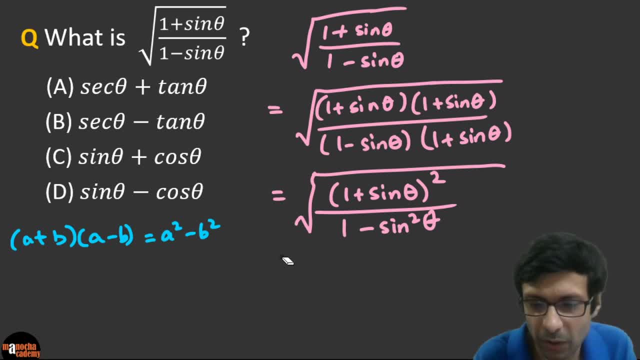 plus. so let me continue it on this side. so let's write this here, so i'll erase this relation. so what we get here, guys? so we are going to get square root of: oh sorry, so it's going to be the square root of the numerator, right? so that's basically square. 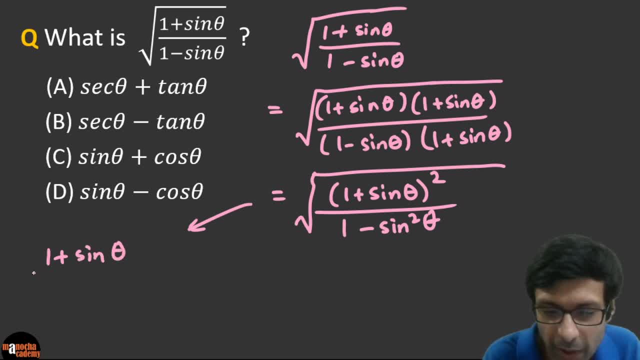 root of the square. so we're going to get 1 plus sine theta there, simple right, and the denominator will be square root of 1 minus, because the square root and square gets cancelled: 1 minus sine square theta. now can you tell me what is 1 minus sine square theta? so let's use our formula. 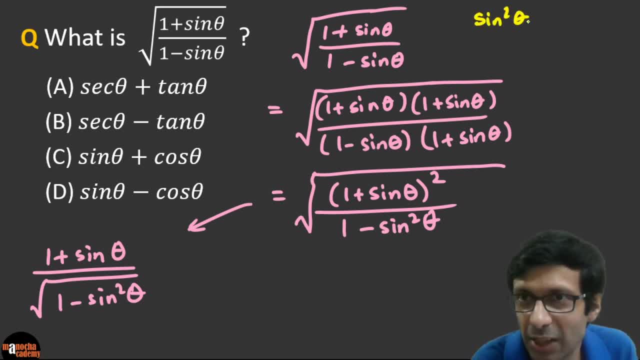 guys, let's use this formula: what is the connection between sine square theta plus cos square theta? oops, so sine square theta plus cos square theta is 1, right, guys? so therefore we can say: cos square theta is nothing but 1 minus sine square theta, right? so can you see that this? 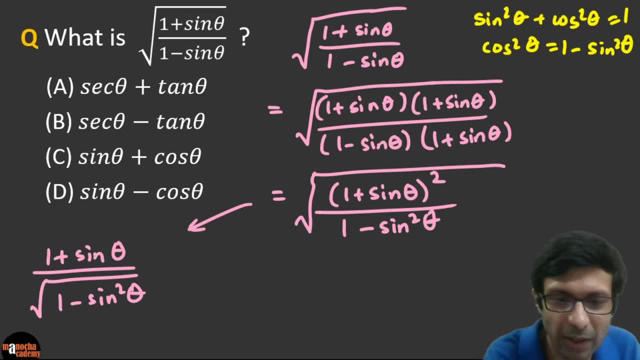 entire term is going to change into: so this is nothing but cos square theta. so what do we have here? so this is 1 plus sine theta divided by square root of cos square theta. do you guys agree? and so that's going to be 1 plus sine square theta. so that's going to be 1 minus sine square theta. 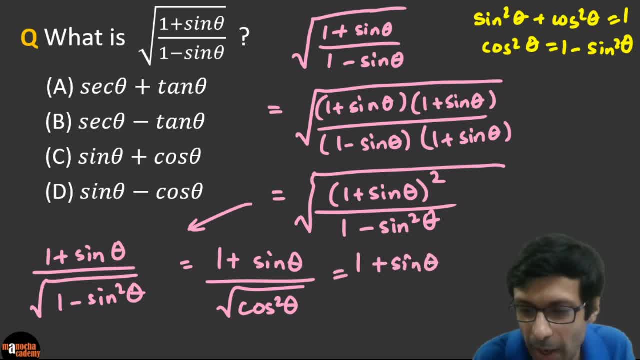 right, so can you see that this entire term is going to change into? so this is nothing but cos square theta, And so that's going to be 1 plus sine theta by cos theta. okay, So all good till here, simple right. And so what do we get finally? 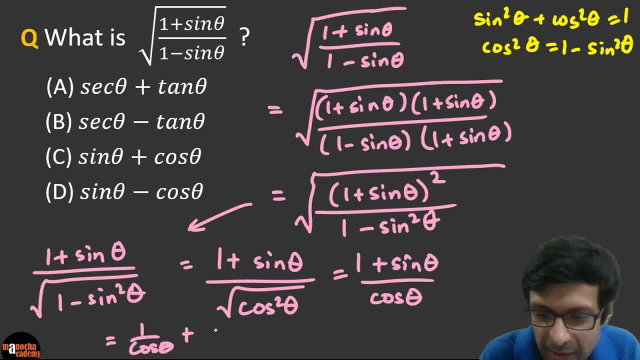 So that's going to be 1 by cos theta plus sine theta by cos theta, right, Okay, and what is 1 by cos theta? It's nothing but reciprocal of cos theta. sec theta plus sine theta by cos theta is nothing but tan theta. 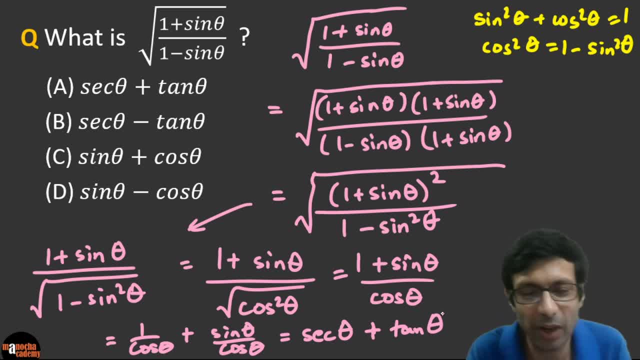 So just a little bit of working, you know, Just doing the step. So the main trick was in the first step. You just multiply by 1 plus sine theta so that this numerator becomes simple, And then we change the 1 minus sine square theta to cos square theta. 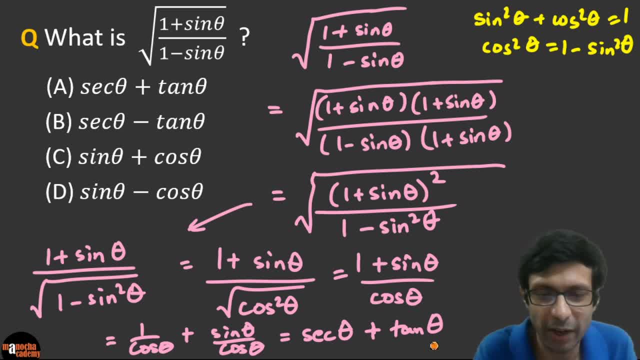 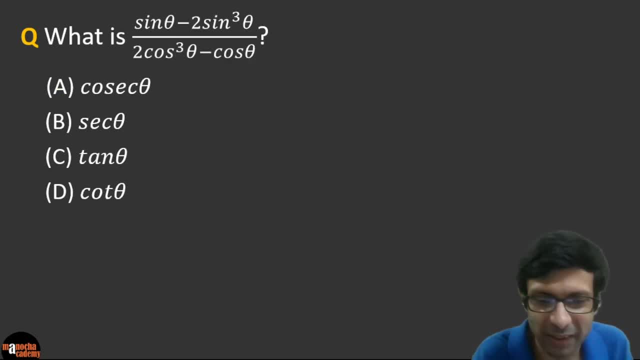 That was the main step here, And after that it's very simple. So, very good guys, The correct answer is going to be sec theta plus tan theta, which is our option A here. Okay, excellent, Let's try this question also. 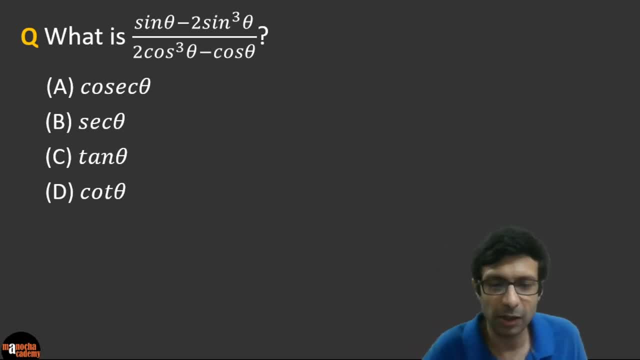 So what is sine theta minus 2, sine cube theta divided by 2? What is cos cube theta minus cos theta going to be? So this one looks a little complicated, but don't worry, Once you start simplifying things, it actually becomes easier. 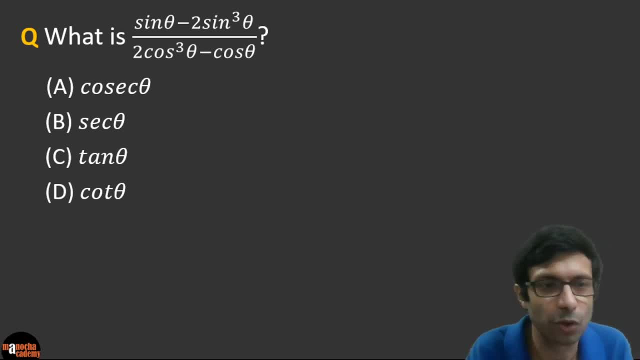 So I want all of you to try this again on your pen and paper, right? So try it out, guys. Yeah, I see some requests for some topics, So guys do write it in the comments. I do read your comments and I'll try to take. I may not be able to take each. 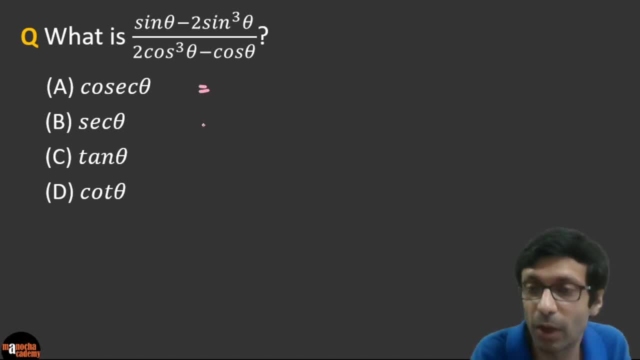 and every topic, but I'll definitely try to take the ones that are popular. you know that a lot of people are asking So very good, So I want all of you to try this question now. So let's see what is this question. 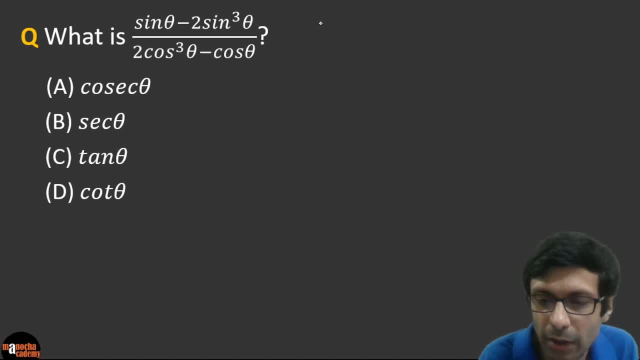 So if you look here we've got, basically we are starting off with sine theta Minus 2 sine cube theta, Right Divided by 2 cos cube theta Minus cos theta. So let's see what we can simplify this to. 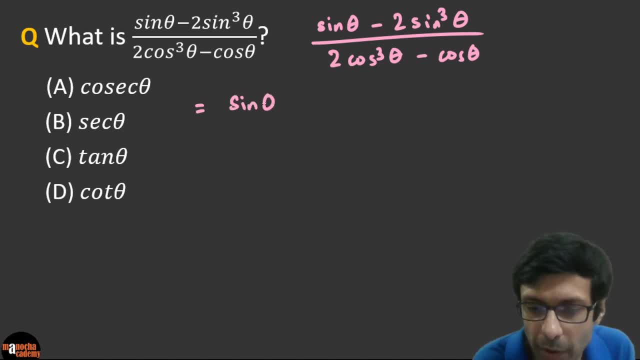 So here you can see that For the numerator let's take sine theta common. So what do we get? 1 minus 2 sine square theta, Simple. And in the denominator we can see we can take cos theta common. So cos theta divided by this is going to be 2 cos square theta. 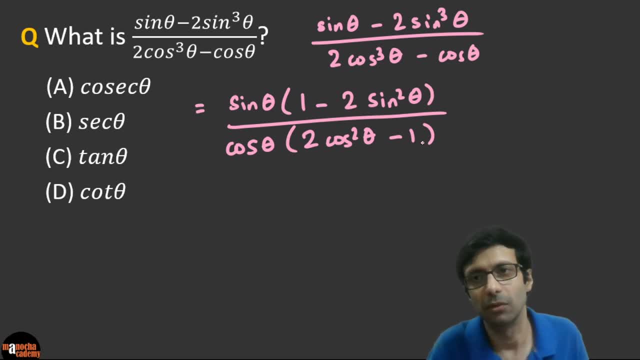 Minus 1.. Right, And guys, you can see, look at the options here. right, Since it's a multiple choice question, you can see the options are very simple. It's going to simplify into: cosec, theta, sec, theta, tan theta, cot theta. 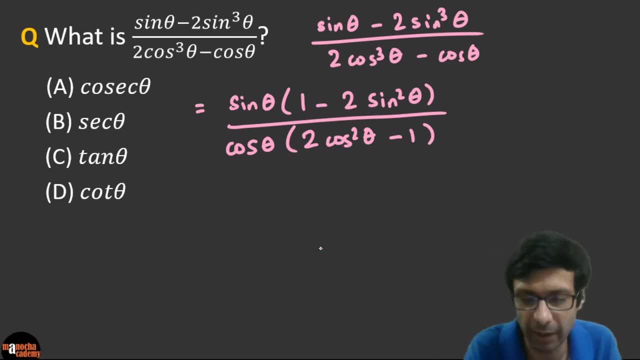 So which one is it going to be? That's what we need to find out here, Right? So it's really simplifying to something really simple. So let's see what we can cancel out or what we can do here, Right? So let's try this out. 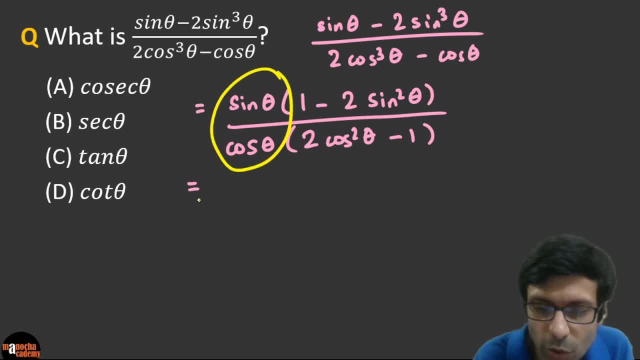 So we know this. Can you see, guys, that sine theta by cos theta. So this is simply going to be tan theta, Right? So this part is very simple. So we have tan theta, and then we have all this fancy stuff here. Right, 1 minus 2 sine square theta divided by: 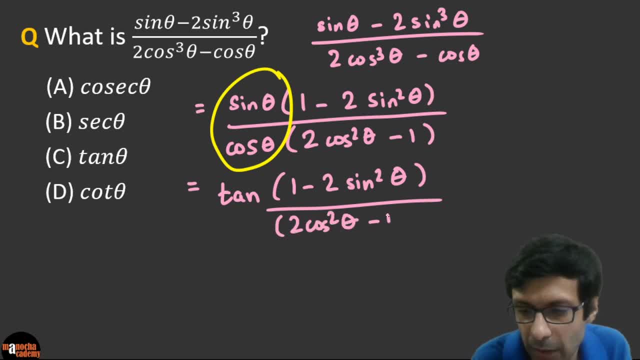 2 cos square theta minus 1.. Guys, can you see that? Okay, So now you can see: in the numerator there's a sine square theta. In the denominator there's a cos square theta. So you can see that there's square, guys, Right. 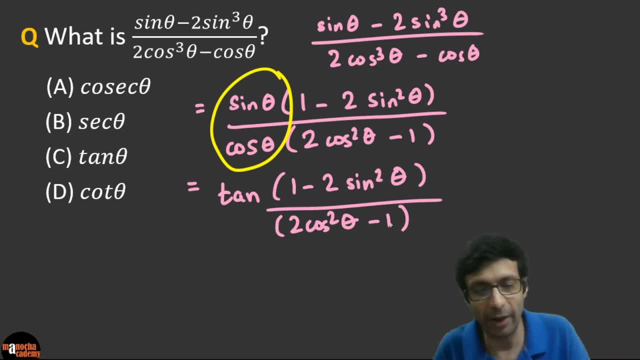 So we need to use our trigonometric identities, the square relations, And what is the important square relation that we learned between sine and cos theta? It was sine square theta plus cos square theta is 1. Right. So that is the important relation that we learned today. 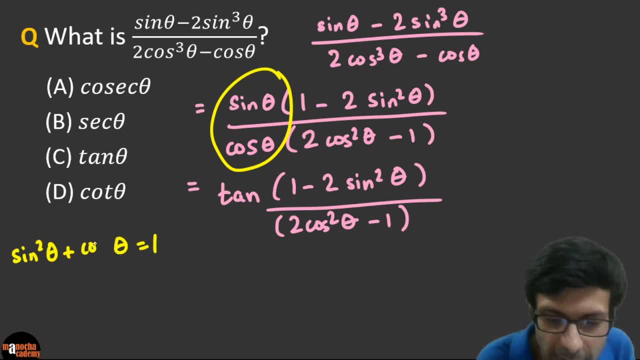 So sine square theta plus cos square theta Is 1.. Right, So let's go ahead and change one of the guys Right? Oops, And I forgot to write. this is tan theta, right? Not tan tan of theta. Okay, So this is going to be tan theta. 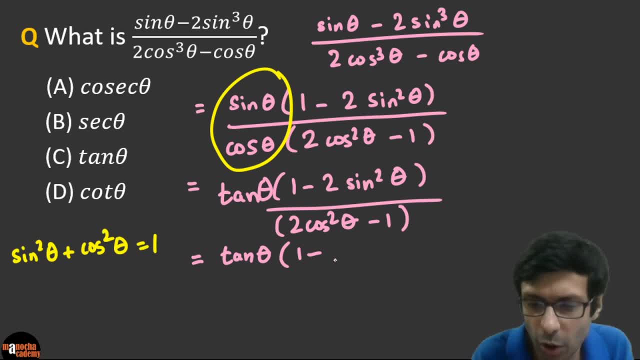 And this one: let's change the sine, let's say to cos. So what are we going to get? So instead of sine square theta, I'm going to put 1 minus cos square theta. So look, this term, this term, on top. 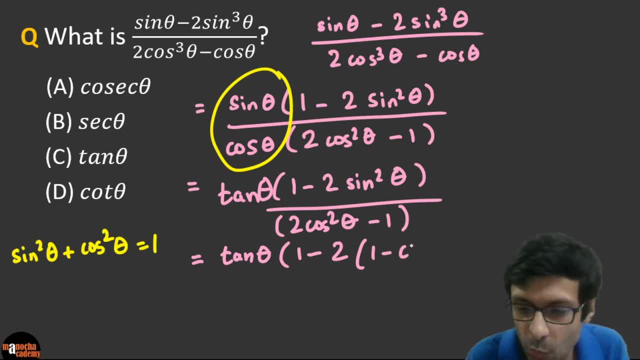 I'm going to substitute- because sine square theta is nothing but 1 minus cos square theta- from this identity. Okay guys, simple, And we're going to keep the denominator the same: 2 cos square theta minus 1.. Now, why am I doing it? 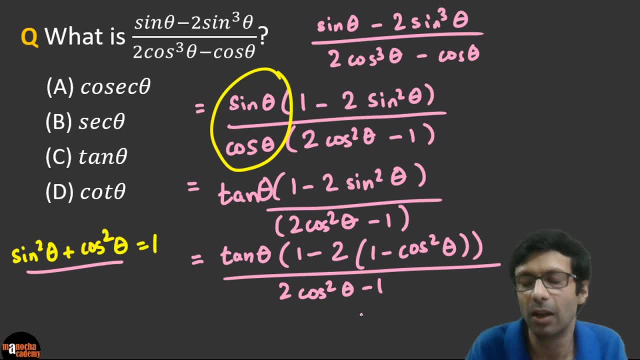 Because we are trying to change sine to cos, So maybe some things will cancel, Right, So you change one of them, not both. Okay, And what are we getting here, guys? So let's see what does this part simplify to? 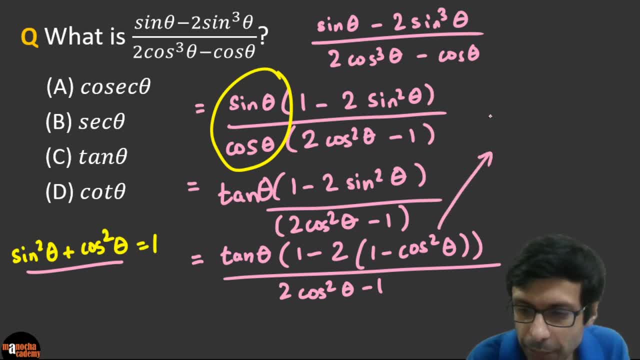 So we are just focused on this part, So we basically get here. So if we look at this part, we have 1 minus. So what do you guys get here? 1 minus 2.. And that's going to be a plus 2. cos square theta? 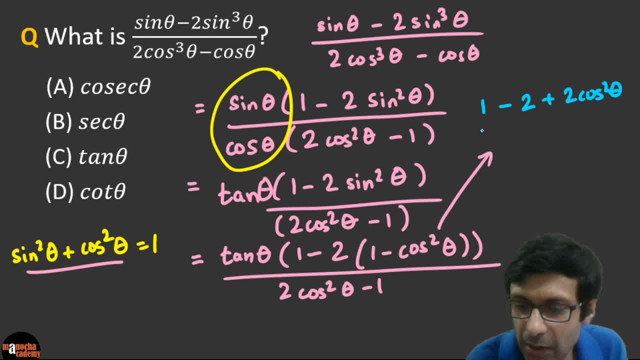 Right. Can you see that? I'm just expanding this. So what am I going to get? 2 cos square theta, Right? So 2 cos square theta minus 1.. Okay, that's really good, because can you see this part? 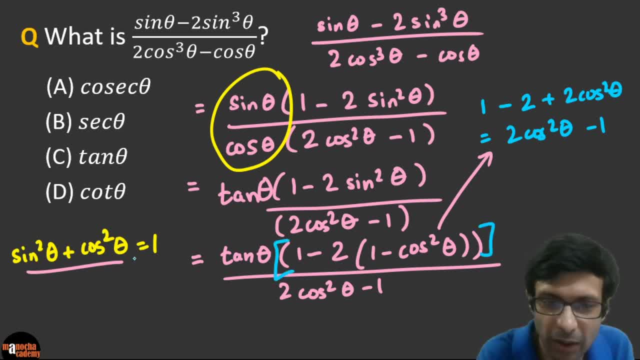 So I was simplifying this part here right in the blue color. So can you see, guys, what are we getting here? So we've got basically tan theta multiplied by. So let's write it in blue. We simplified that bracket portion to 2 cos square theta minus 1.. 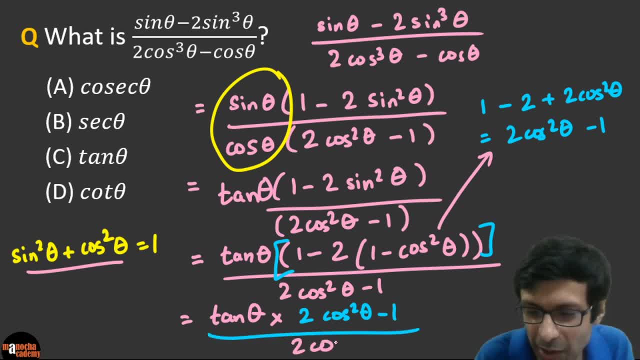 And the denominator is also 2 cos square theta minus 1.. Yay, So that's great. Now this and this will cancel, Right guys, So we can cancel this part. These are going to get canceled, And what are we only left with? Tan theta. 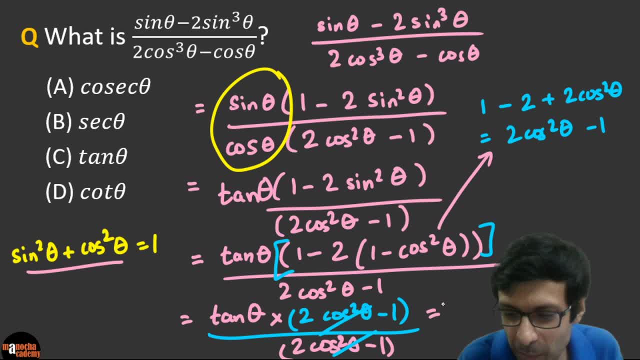 Excellent, Excellent guys. You guys got it Superb. So nothing great here, No rocket science, Basically, look at the thing you saw. We did the simplification, took out sin theta, cos theta. Now you see the square relation. 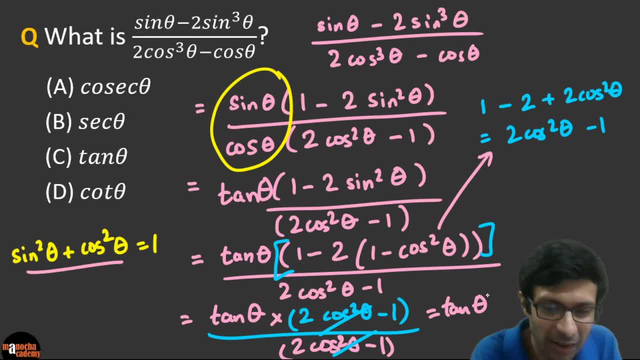 So those cubes changed into square. That means you need to apply our trigonometric identities. We use this formula, right? We use this formula and applied and simplified it, And so see it worked out to such a simple thing. So once you practice, guys, so please watch this video. 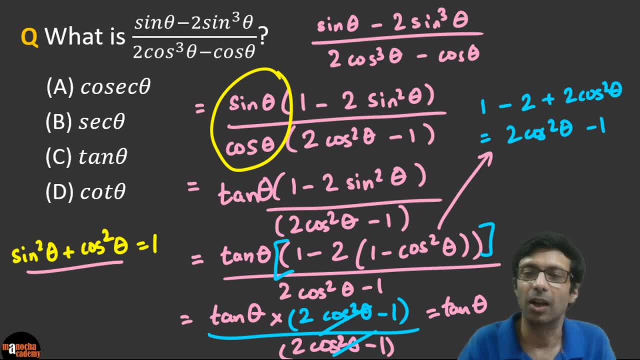 And you can also watch my video on the basic trigonometry, which is on our YouTube channel, And then you'll find all of these questions much easier with practice. So it's just a bit of practice and learning up your formulas. And I have one homework question for you to practice. 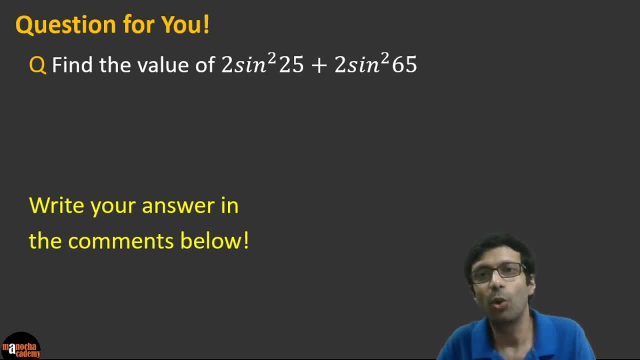 So, guys, this question is for you: Find the value of 2 sin squared 25 plus 2 sin squared 65.. So 25 means 25 degrees, right, And 65 degree. So this is the question for you, guys. 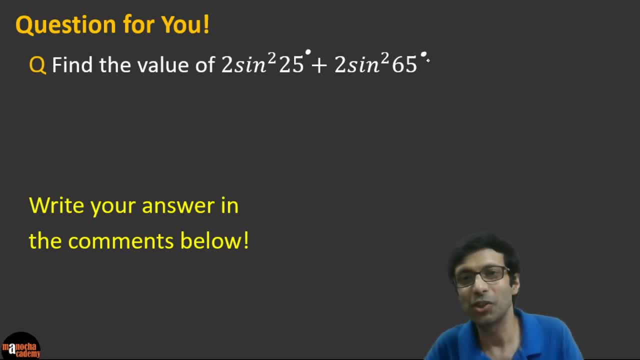 And I won't discuss the answer here, because this is our homework question And I want all of you, each one of you, to try this and write down the answer in the comments below, And I'll definitely take a look at your answers. 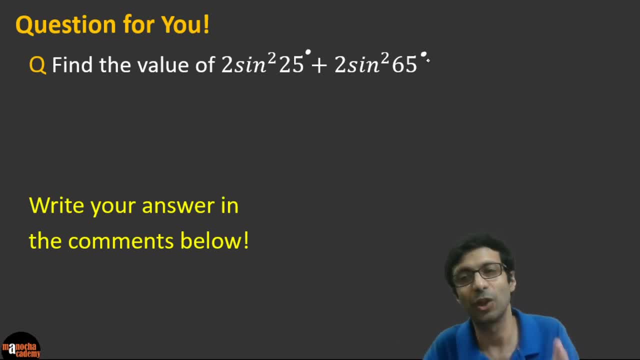 And you've seen that I've tried to reply to your answers for the homework questions as soon as possible. So, guys, please try this out, OK? so please go ahead and take a look at this question: 2 sin squared 25 degree plus 2 sin squared 65 degree and apply the concepts. 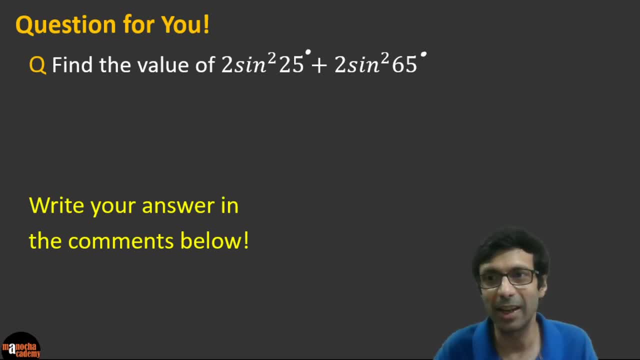 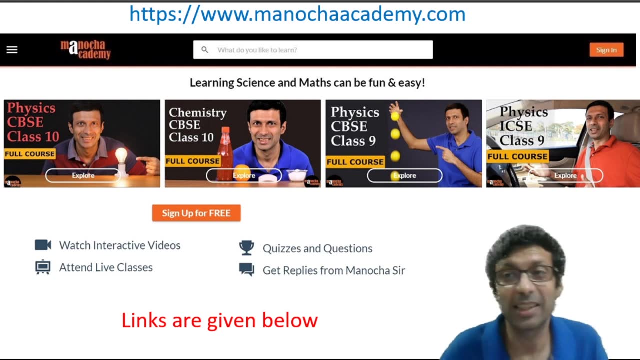 that we learned in the class today. So we learned about trigonometric identities and trigonometric ratio of complementary angles. OK, so please try it out And, guys, as I said, do check out our awesome courses on physics, chemistry, and soon we are launching the maths courses as well. 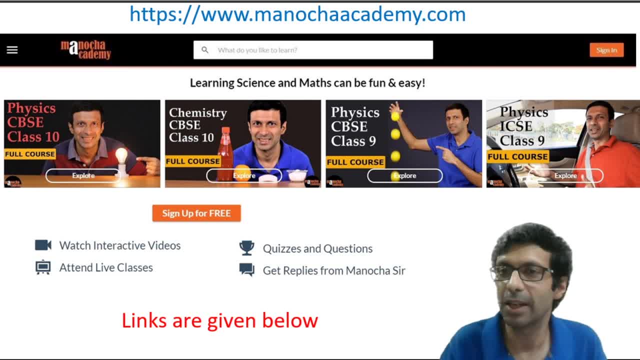 And these are all to help you with your preparation for CVSE. And we have the physics ICSE class nine course Also. the links are given below and we have really big discounts for a limited time, So guys do check them out. 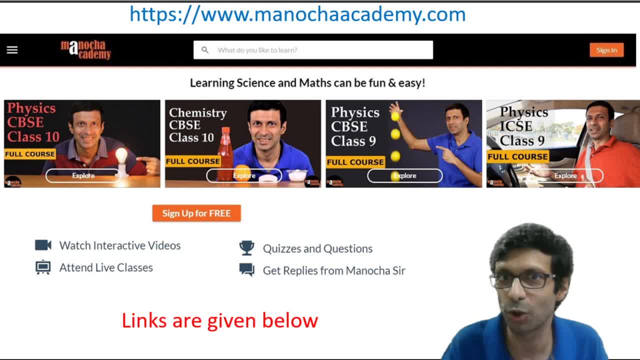 I think you'll find them very useful and have special life classes also, which I'm taking. those special life classes quizzes and questions and you get to watch interactive videos. So this is to help you guys with your preparation And I hope all of you are studying and making use of this lockdown time where I 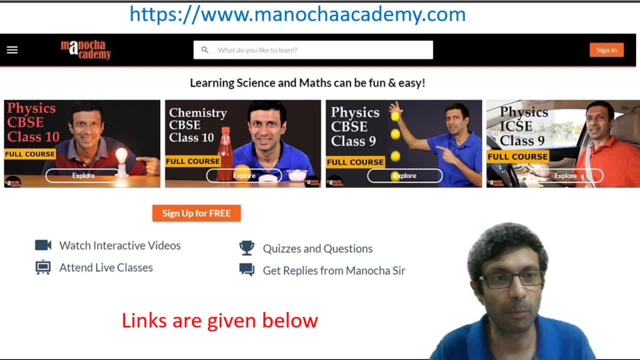 know all of us at home, it's a very difficult time, So I pray for everybody's health. Guys, please take care of your health and family, Stay safe, stay positive and keep on studying, guys. That's my message to you. 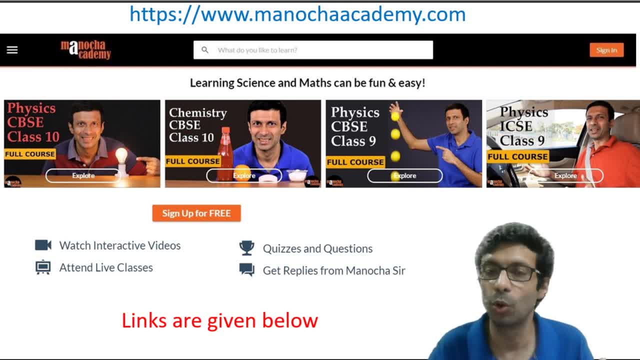 Please keep on studying and practicing and also use your textbook for more practice And do check out our courses. And if you haven't subscribed to our YouTube channel, what are you waiting for? Please hit the subscribe button right now, Like this video and please share it with your friends.